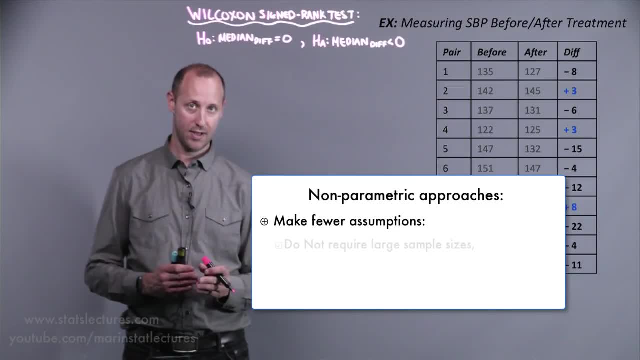 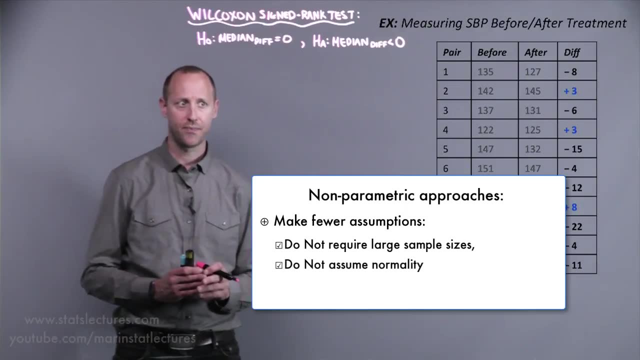 But one of the pros of these is they make fewer assumptions, They don't require large sample sizes, They don't assume normality. So that's kind of the nice side of them And also a reminder: aside from non-parametric approaches, we could work with bootstrapping or 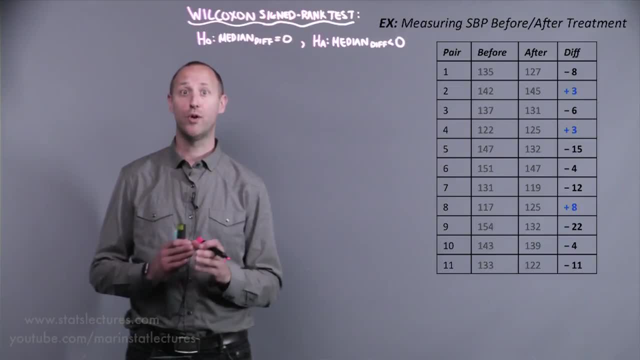 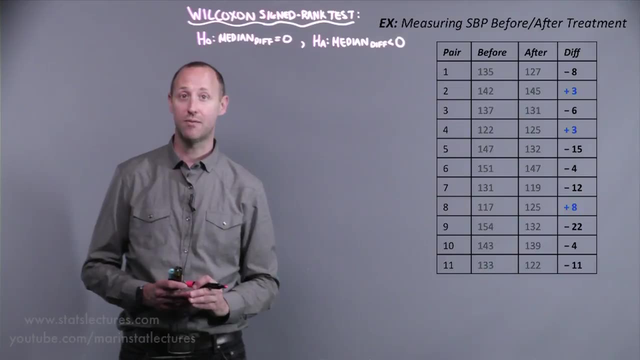 resampling type approaches if we don't have large sample sizes or if we don't want to make as many assumptions, normality being one of them. So we're going to work our way through this way up to the Wilcoxon signed rank test, And while we're going to do some of the calculations, 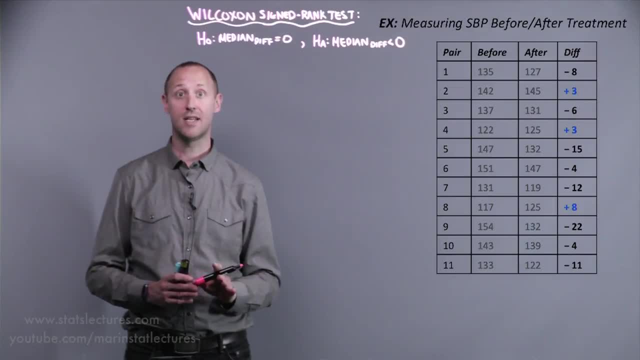 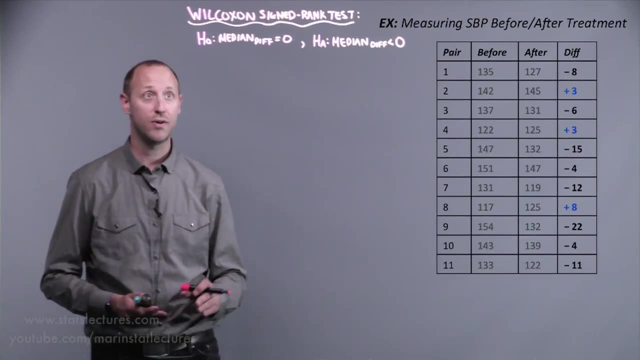 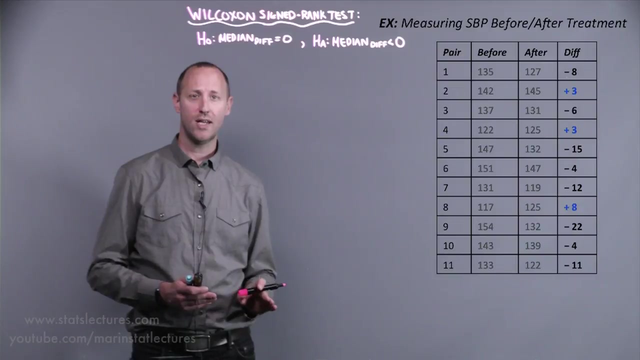 we want to focus on the concept underlying this test as well as just non-parametric approaches in general. So recall the parity test we were testing: is the mean difference zero? And here we're going to get at the median difference. And before getting into the Wilcoxon signed rank test, 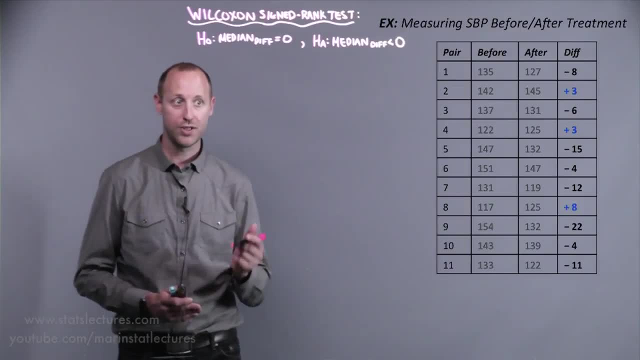 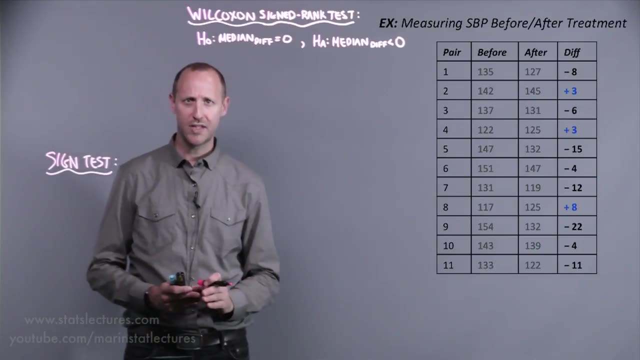 we're going to start with the simplest form of a non-parametric approach, The sign test. And this test is probably a little bit too simple to be useful, but it's a good building block for what is a non-parametric approach. So this tests the same null and 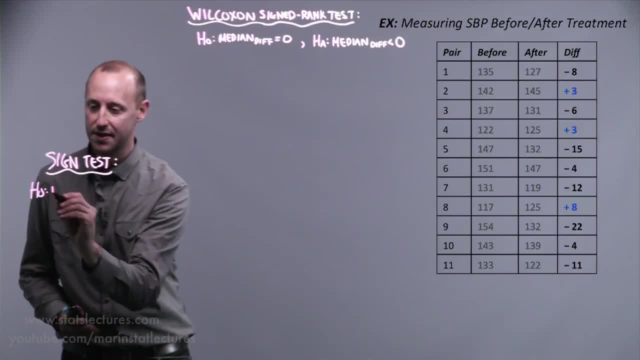 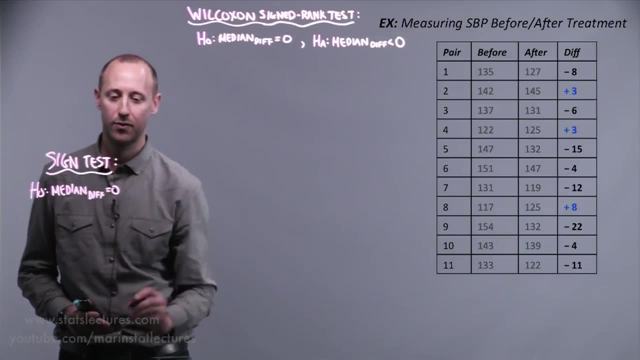 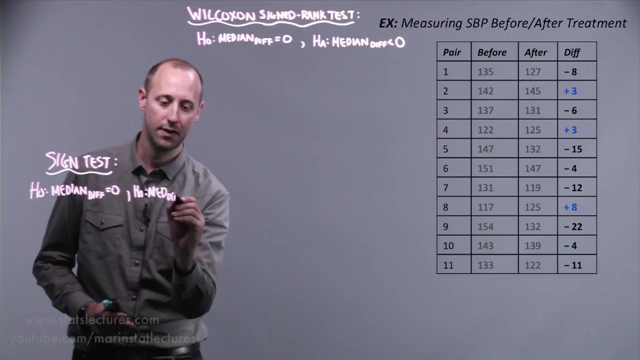 alternative Tests, a null hypothesis that the median difference is zero, versus an alternative that the median difference is zero And we're going to get at the median difference And we're going to get from here to this situation. Let's try this one. So this is a non-parametric approach. 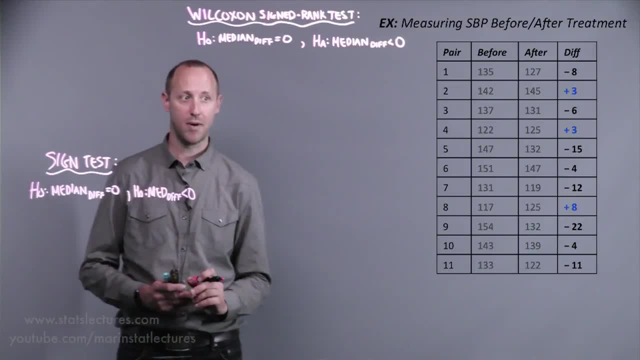 Same study, Same hypothesis test, And let's see: either X is zero or is that zero, Someone had a less than one. We get a sign then And then say: you test for the negative, in total it might be minus 0. So this test are doing what it's right now, And so after you write, 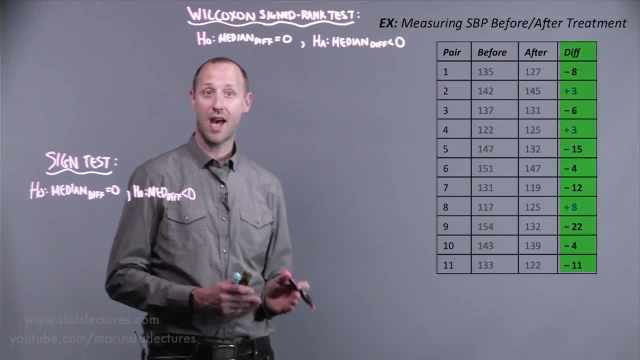 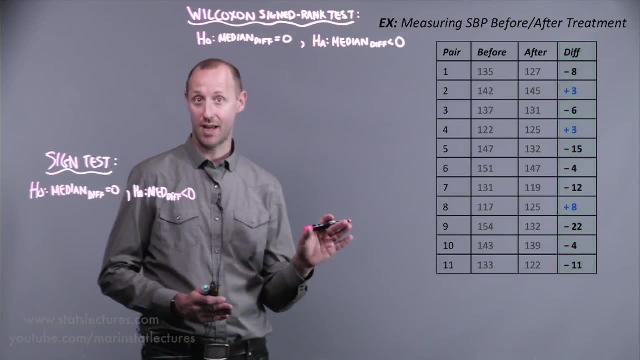 down your Nevertheless Zombies. it's going to look so simple And in other languages, the damages between difference for value 0 and minus 0 is less than zero if the greater or the greater value gap is less than 0. So some people had increases, some people had 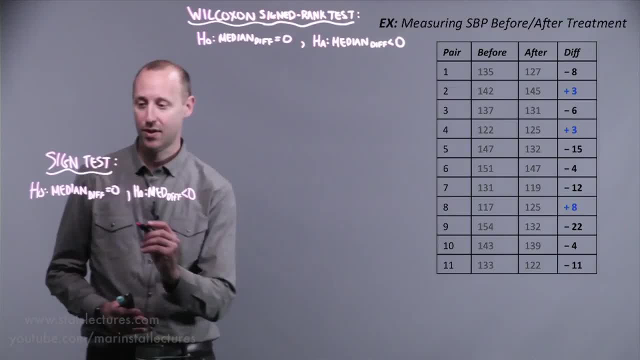 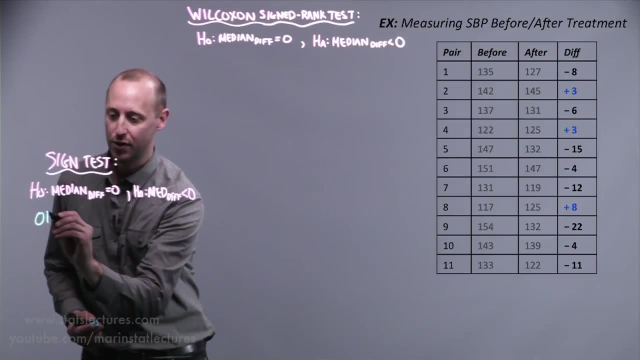 decreases, And so we've been kind of zast Higher, refreshed blonde figure scene now. But let's go back to the portfolio market. So, basically, this is just another test. enjoy, let's, let's change our color here. we'll see that what we've observed 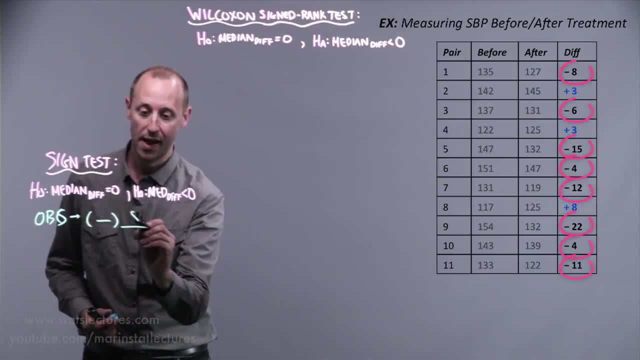 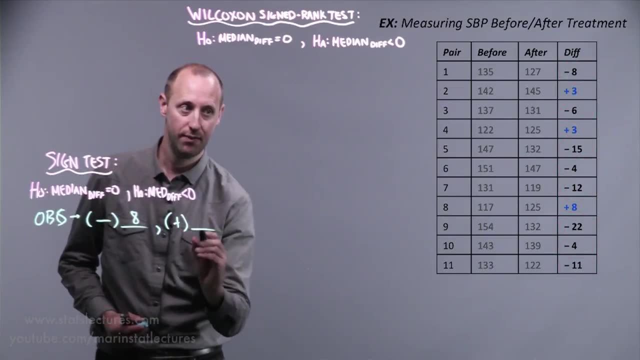 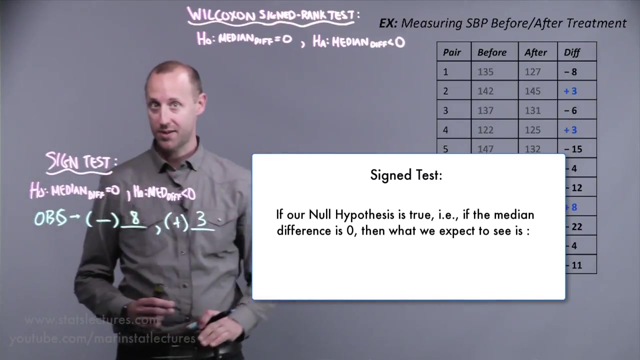 is that for the decreases, there were eight individuals who experienced a decrease in the systolic blood pressure after treatment, and for the increases, we count them up, there were three. now what the sign test does. it says, if our null hypothesis is true, right, if the median change. 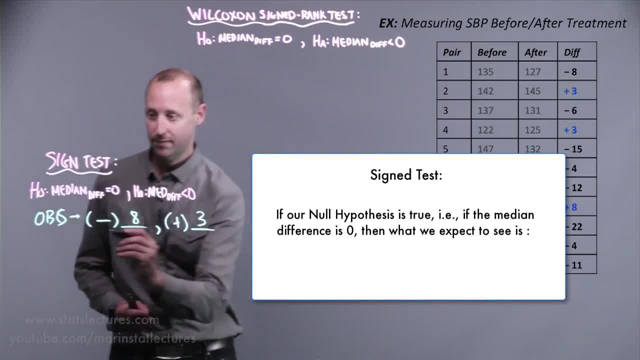 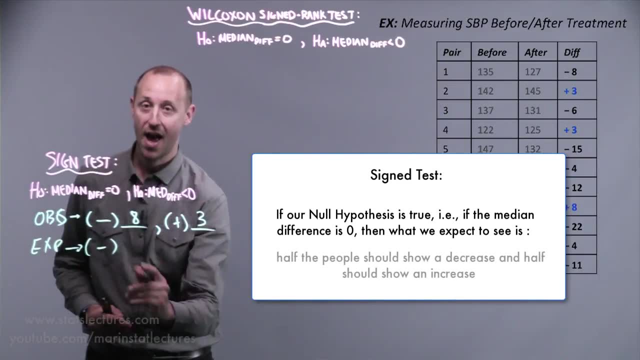 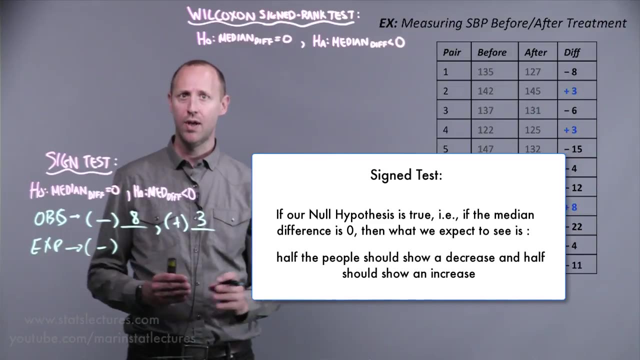 or the median difference should be zero, then what we'd expect, what we'd expect to see if our null hypothesis is true, is that half of the people should show a decrease, have to show an increase, right, if there's, in theory, no difference between before and after, we'd expect to see some people go up, some go down, and it to be about a 50: 50 split. 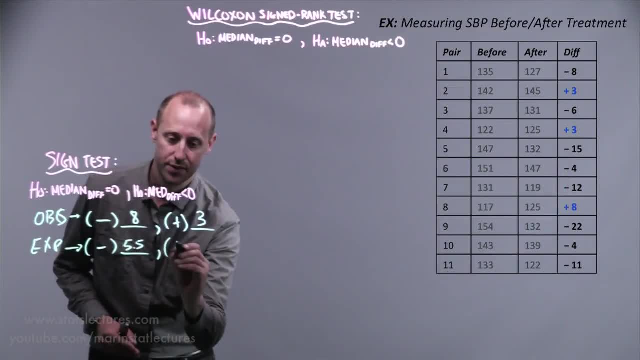 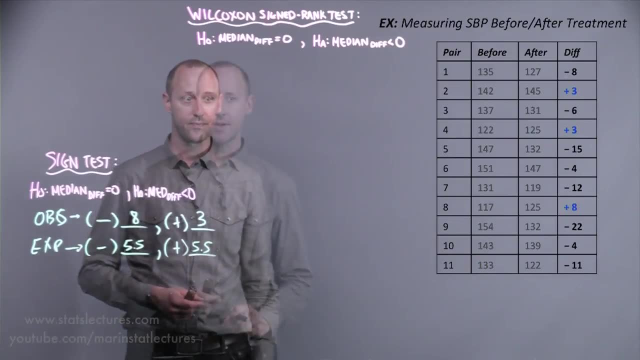 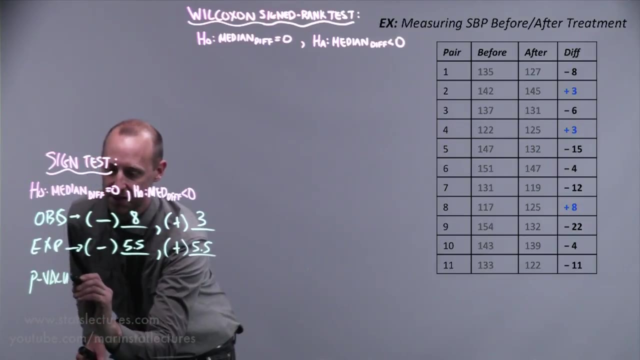 so we'd expect, out of our 11, five and a half to show a decrease and five and a half to show an increase after treatment. so now we can work out the p-value for this and p-values, while the calculation of them changes slightly, the underlying 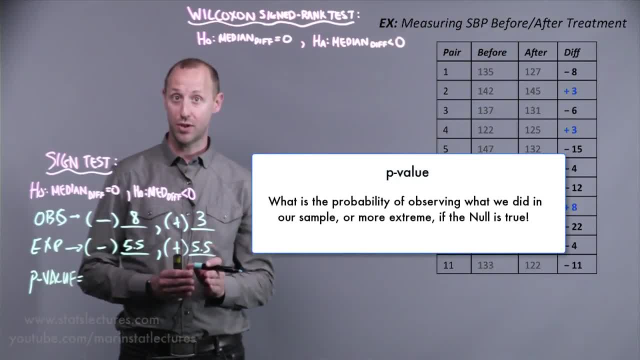 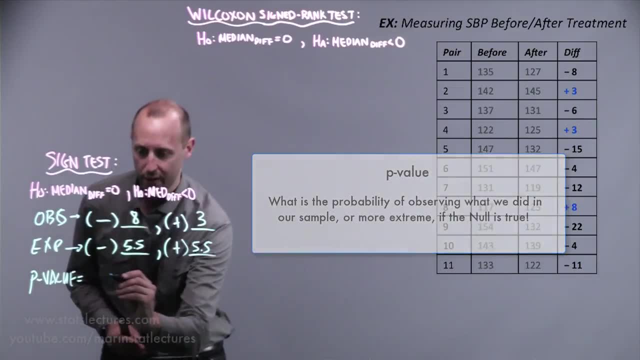 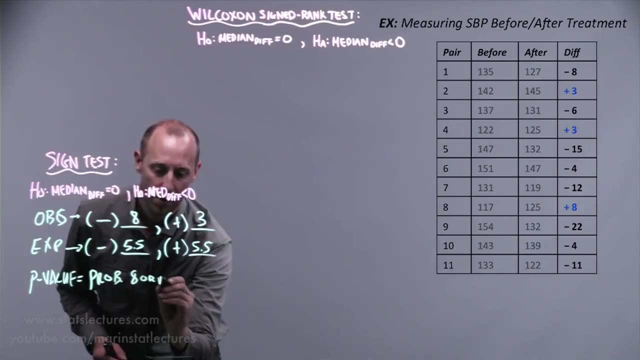 concept is always the same: what's the probability of observing what we did in our sample, or something even more extreme or further from the null, if the null is true? so here we want to work out what's the probability of seeing eight or more- let's just say decreases- eight or more people showing a decrease after. 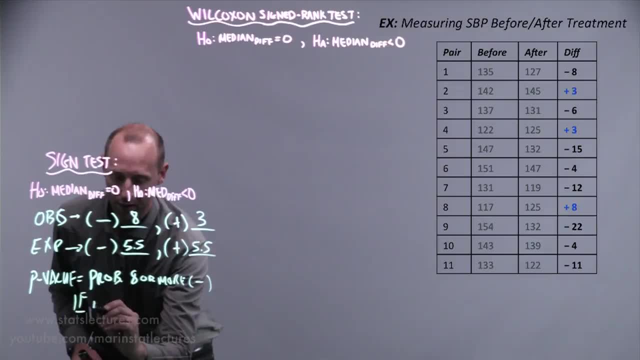 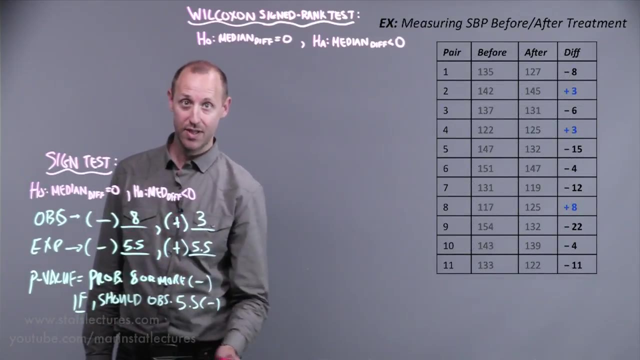 treatment. if the null is true, okay, in that case, if we should observe five and a half, so what's the probability of seeing eight or more people showing a decrease after treatment if, in theory, we should have seen only five and a half? okay, okay, okay. you may build this connection or notice that this follows a binomial. 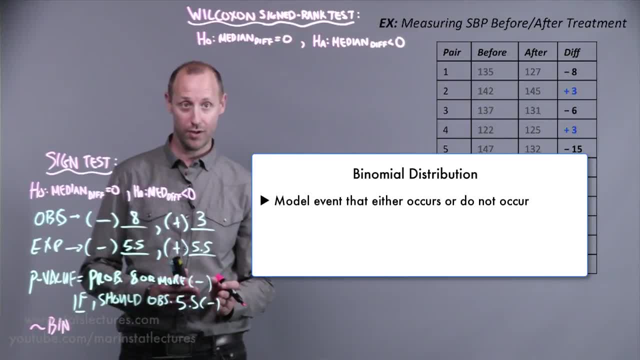 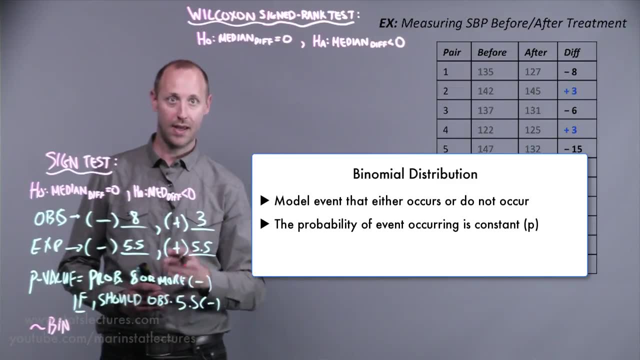 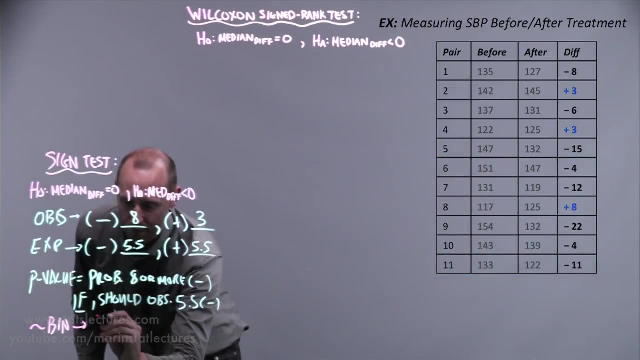 distribution, binomial models, things that either occur or don't occur. right, there's a decrease or there's not a decrease. the probability of a decrease is constant- in this case 50%- and each trial is independent. each person showing an increase or decrease is independent of the others. so here we can work out for a 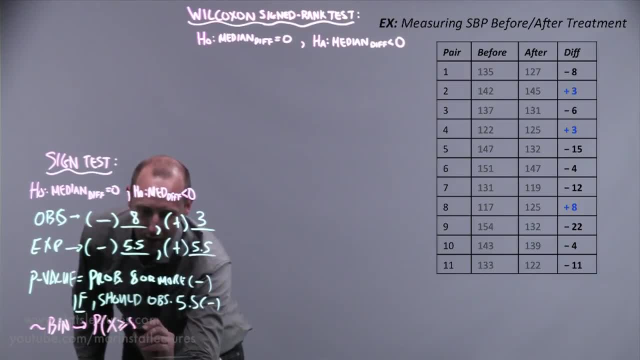 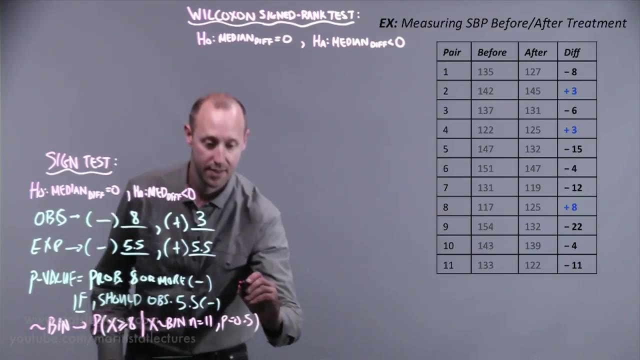 binomial, what's the probability of seeing X greater or equal to 8, given X is a binomial with 11 trials, 50% chance probability of success, if you work this out you're going to find it comes out to be 0.11 or 11%. so there's about an 11%. 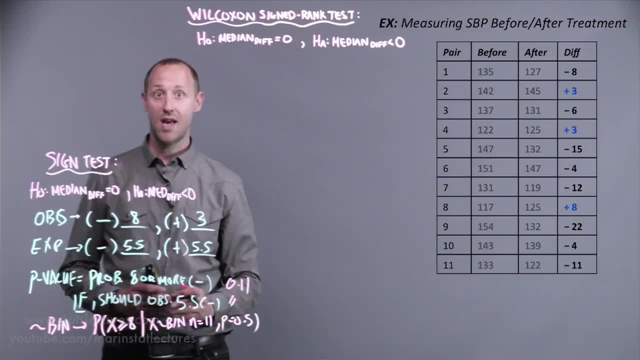 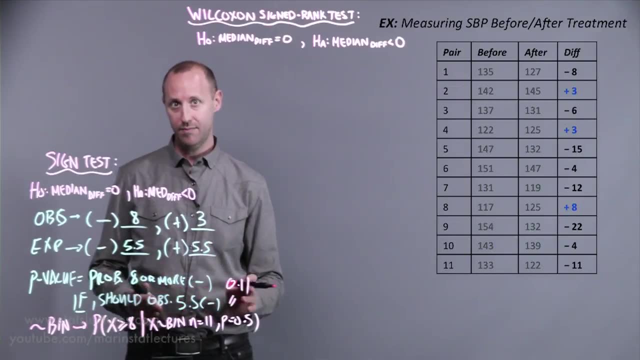 chance of seeing eight or more people showing a decrease, if in theory it should have been a 50-50 split and we should have seen about five and a half care minor. this is the one-sided test. to do the two-sided test, we double that P value. 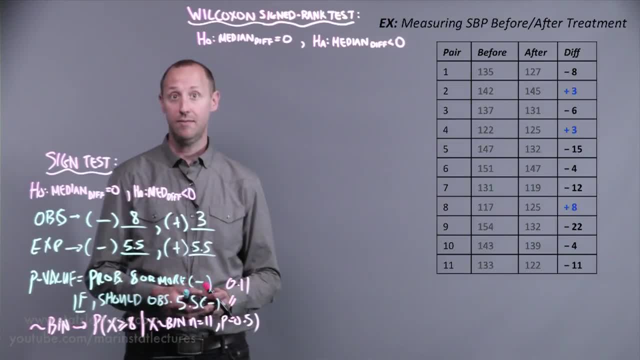 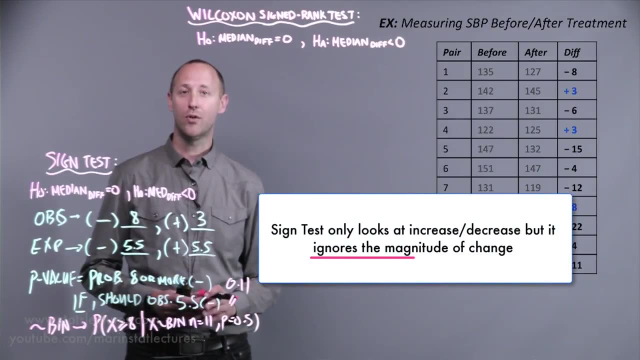 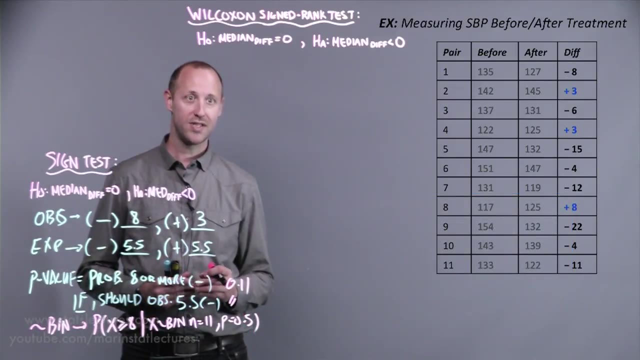 value. But one thing to note about the sign test is it's a little bit simple. It only looks at was there an increase or a decrease, but it ignores the magnitude of the change. So in other words, it treats a decrease of three in blood pressure the same as a decrease of 30. It doesn't. 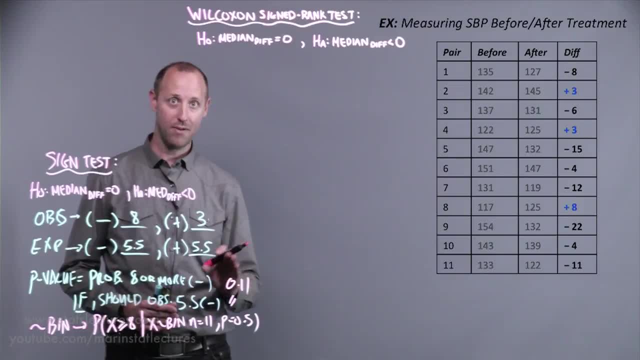 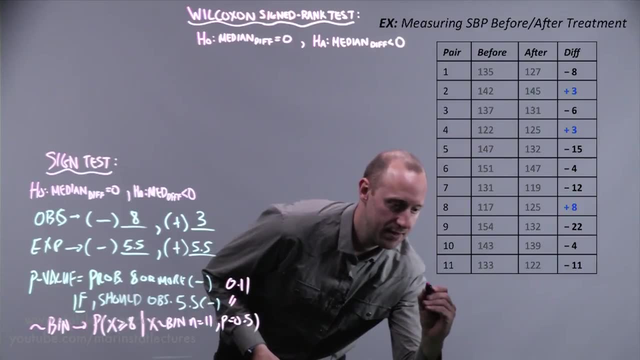 differentiate between those two. We're going to highlight the problem of the simple sign test here. So I'm going to create an exaggerated example. So I'm just going to label this example number two, And we're going to consider a sample size of seven. Again, this is going to be. 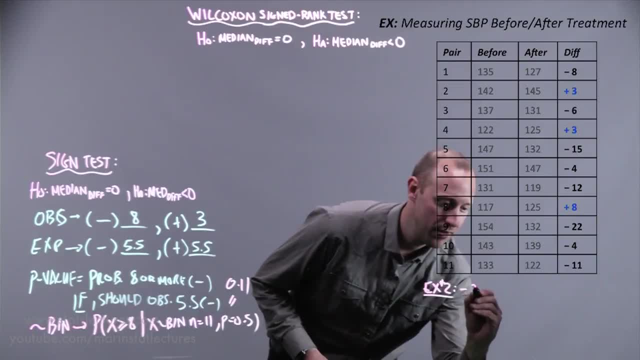 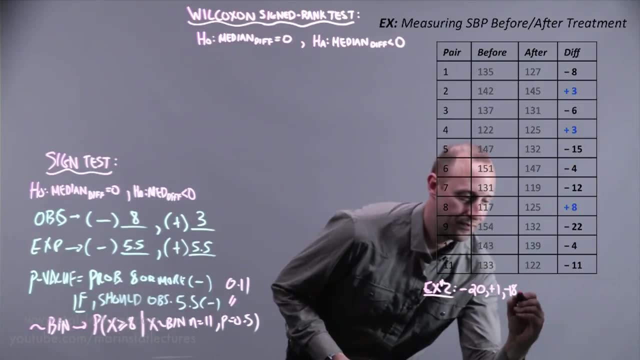 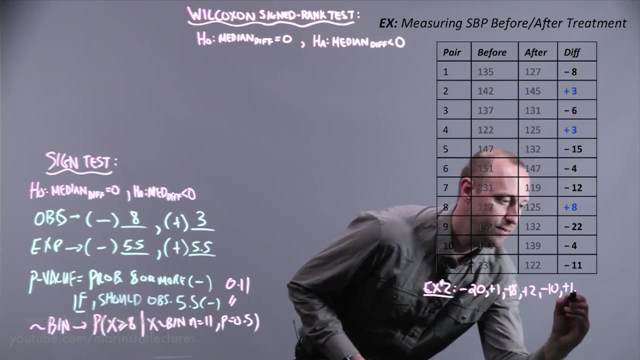 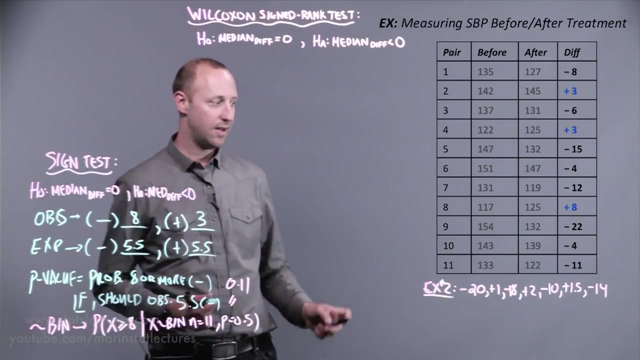 exaggerated. to draw out a point, Suppose we saw someone had a decrease of 20, an increase of one, a decrease of 18, an increase of two, a decrease of 10, an increase of one and a half And a decrease of 14.. One thing you can notice here is that we observed 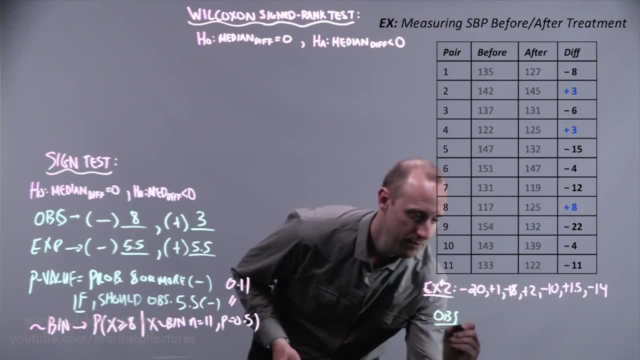 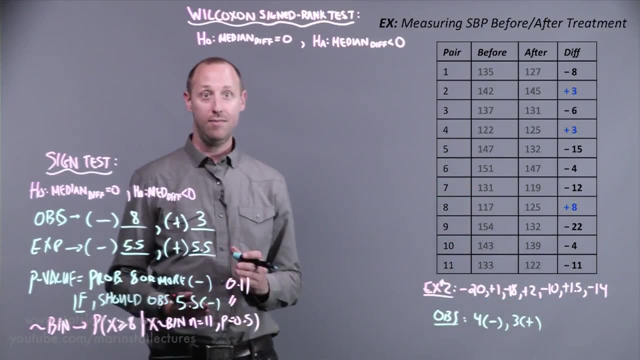 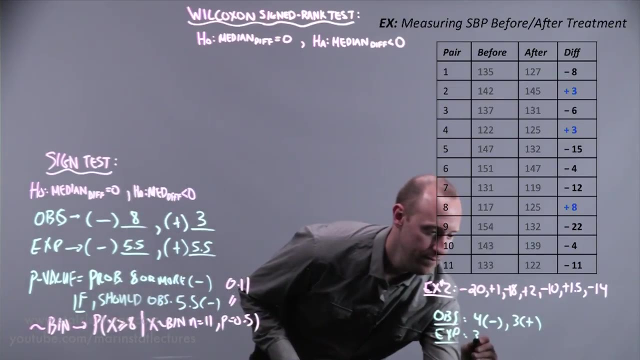 four people showing a decrease, three people showing an increase. And if our null hypothesis is true, what would we expect? We'd expect three and a half people to show a decrease, three and a half people to show a decrease and three and a half people to show a decrease. And if our null hypothesis is true, what would we expect? 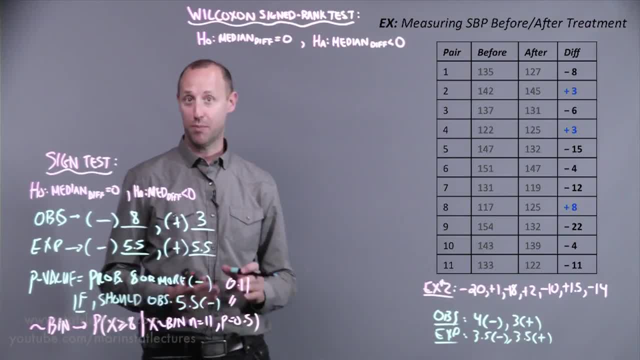 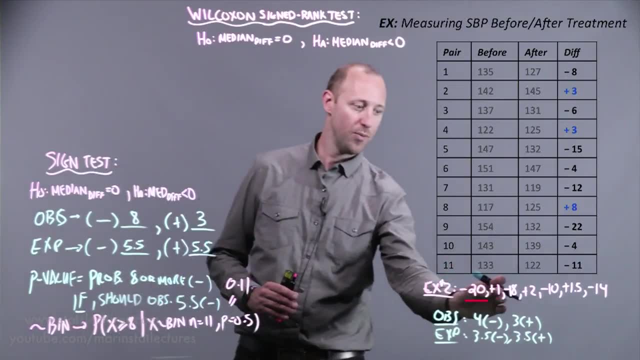 Three and a half people to show an increase. So what we observed is perfectly in line with what we'd expect under our null. But what do we notice here? in this exaggerated example, There are four people who seemed to. the drug seemed to be really effective for them. 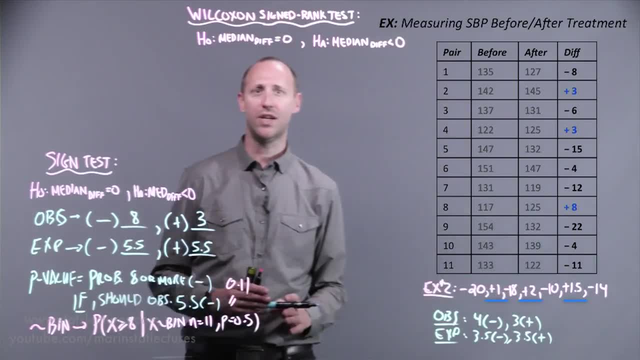 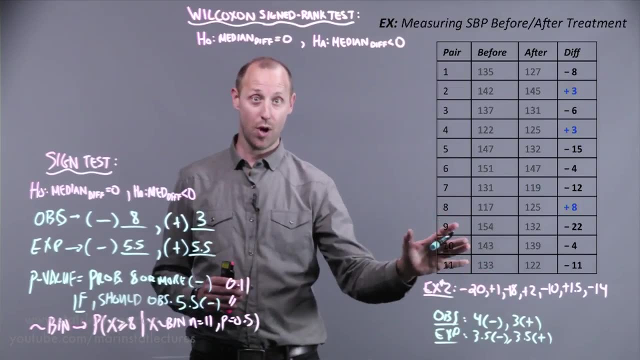 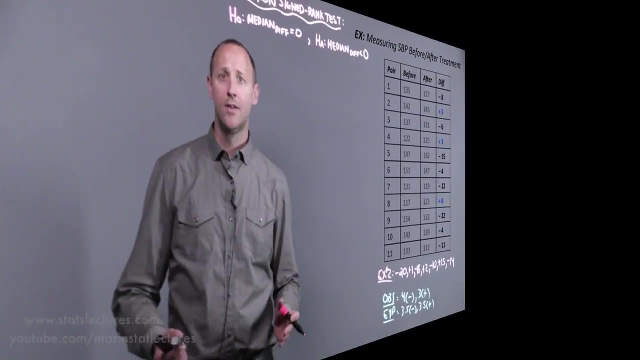 They had a pretty large decrease And there are three people whose increase was negligible. It looked like not much change. So this is an exaggerated example meant to draw out a point. This simple sign test ignores the magnitude of the change. So we saw that the sign test was a little bit too simple. 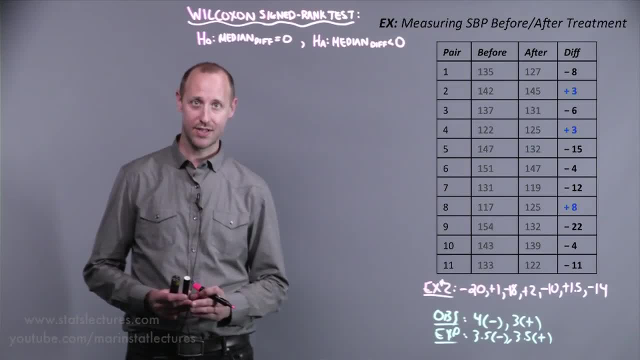 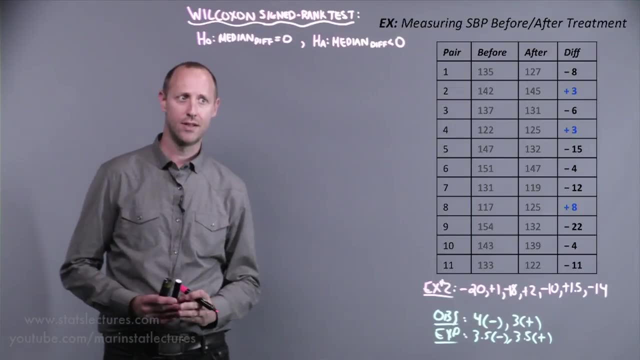 and that ignored the actual magnitude or size the change. So we'll look at the Wilcoxon signed rank test. Okay, so we're going to add in the ranks to the signs. So, essentially, what we're going to do is we're going to take a look at the changes that we've seen. 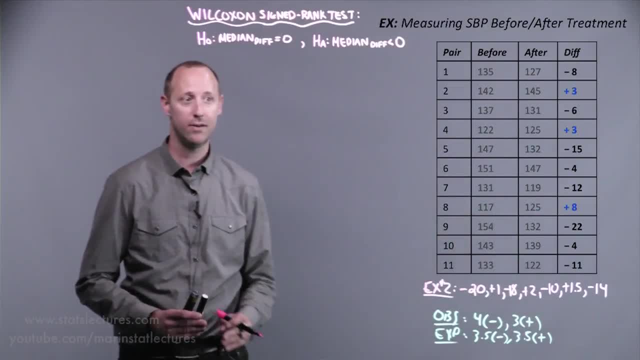 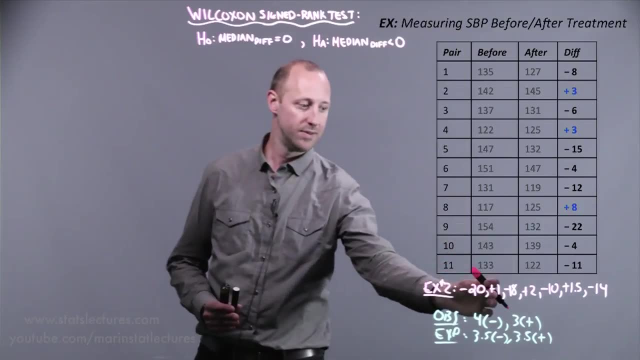 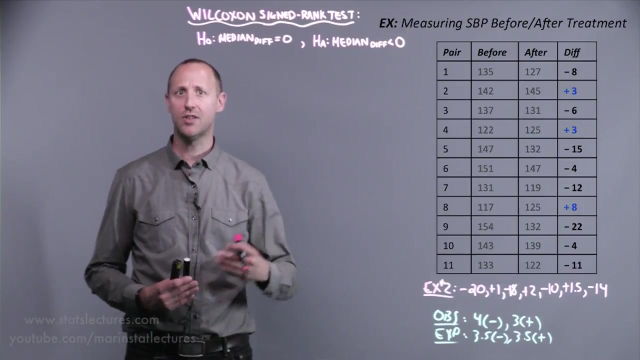 Okay, neither one of these examples- example 2 or example 1 here- And we're going to rank the changes in absolute size or absolute magnitude. So what's the smallest change, What's the second smallest change, What's the third smallest change, And so on, And we can rank them from smallest to largest. 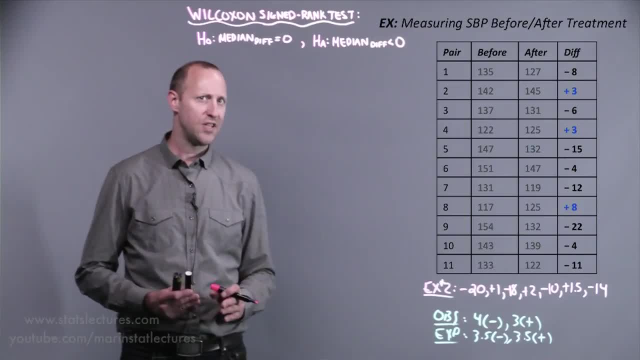 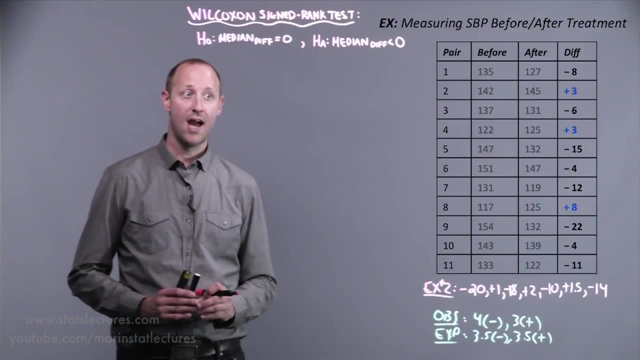 or largest to smallest. It doesn't really matter. Convention is usually smallest to largest, but, like I said, it doesn't make a difference. So what we're going to do is rank the size of the changes, and then we're going to sum up the ranks for all the decreases. sum up the ranks for all the. 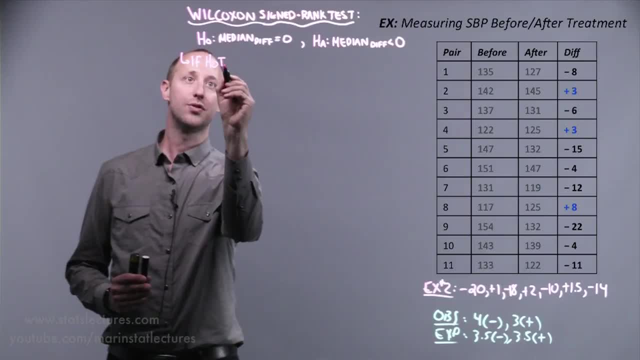 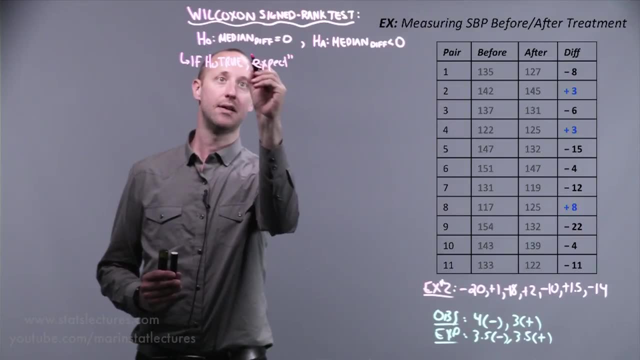 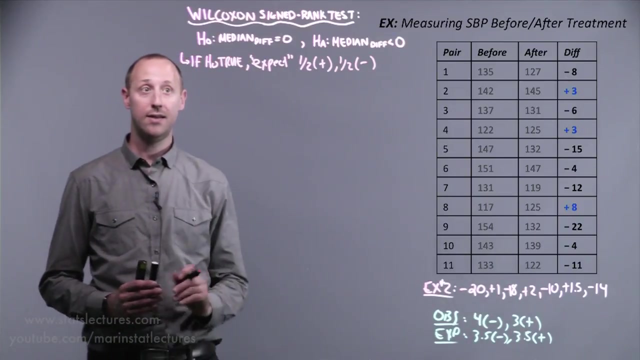 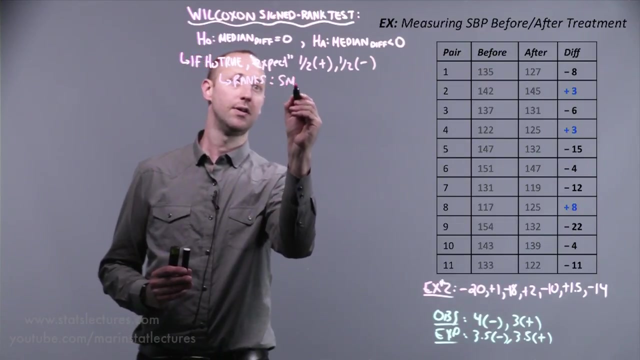 increases and compare those two. If the null is true, we've already noted that we're going to expect about half the people to show an increase, half to show a decrease And, in terms of the ranks, we're going to expect the small. 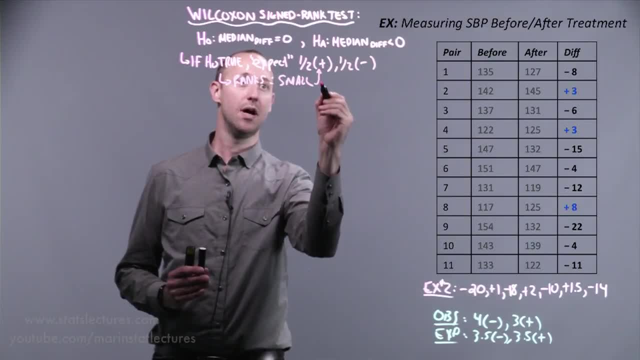 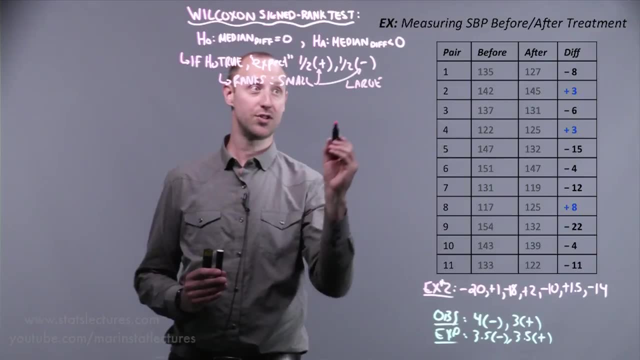 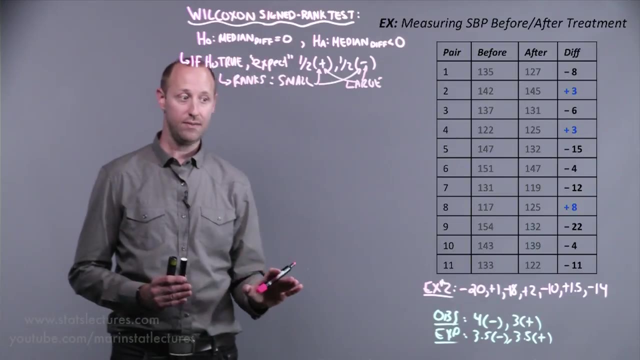 ranks, the small changes to be equally distributed amongst increases and decreases, Same with the large ranks or the large changes. If the null is true, we'd expect to see large decreases and large increases. So let's look at doing this First. we'll do it on our simple example here. 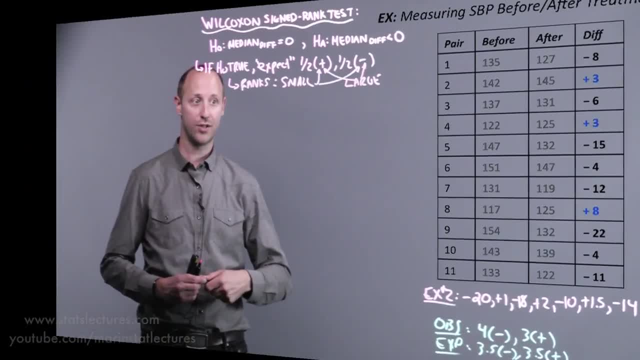 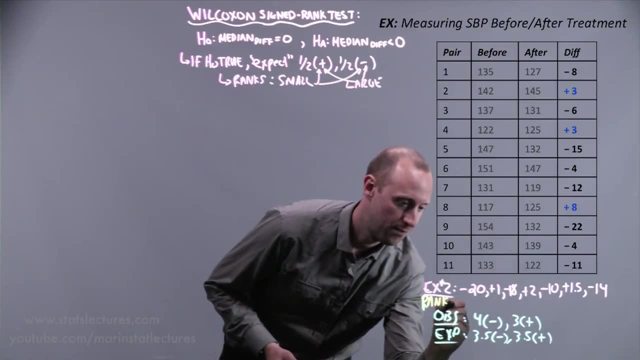 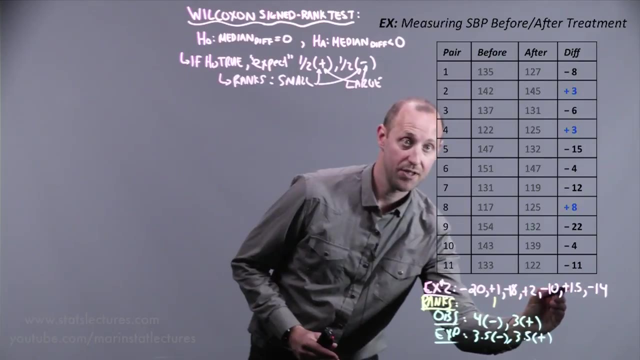 and then after that we'll move to doing it on the slightly larger example. So here I'm going to add in the ranks. So first let's find the smallest change, That's this one, Then the second smallest change, again in absolute value. 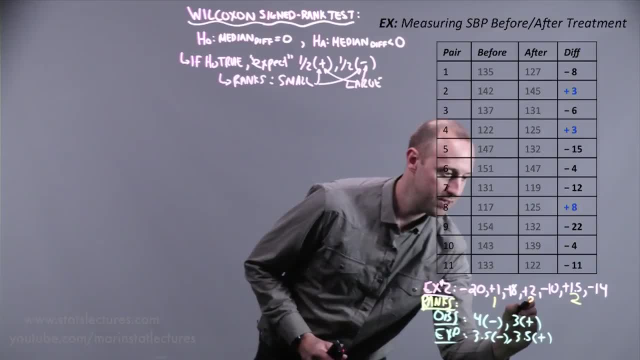 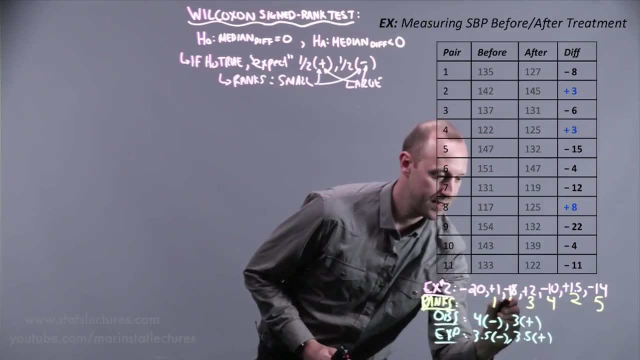 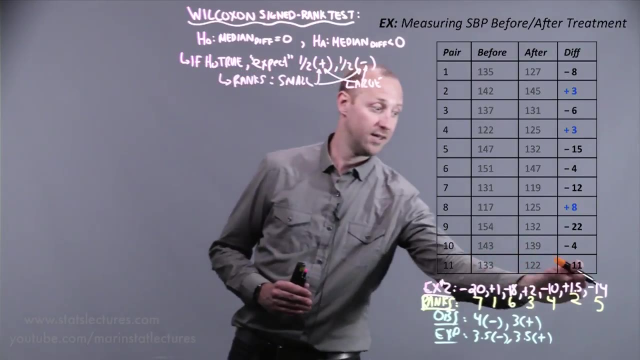 is here The third smallest change, the fourth smallest, the fifth smallest, the sixth and the seventh. And the convention is: if two observations are tied, suppose that there were, say, two decreases of 14, showing the fifth and the sixth rank. we average those two. But again, we don't want to focus. 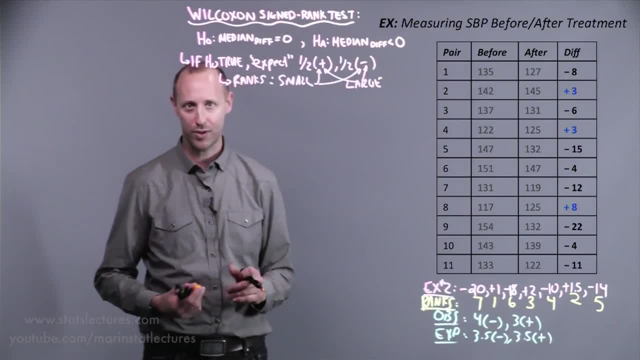 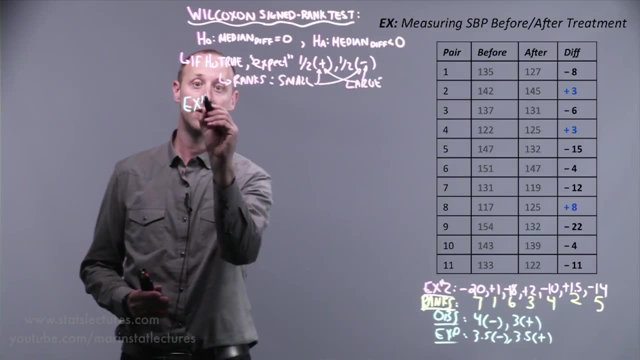 too much on the mechanics. we want to focus on the concept. We can let software do the mechanics for us. So now let's get to first this one here example, what we're calling example number two. Let's talk about what we'd expect. 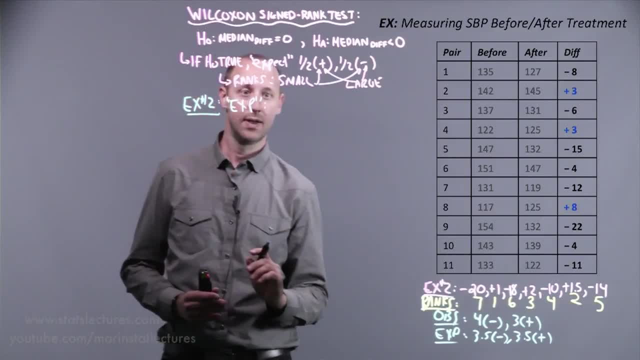 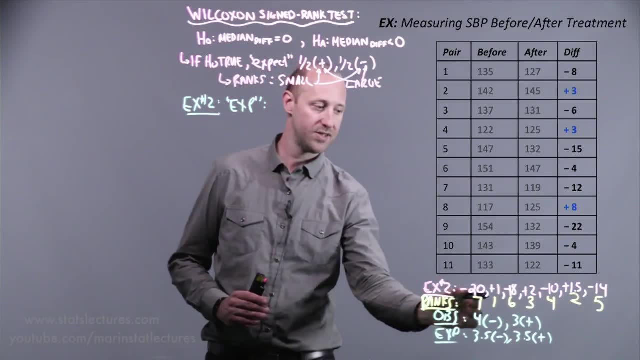 if our null hypothesis is true, We'd expect to see about half the people showing a decrease, half showing an increase. If we sum up all these ranks: one, two, three, four, one plus two plus three plus four plus five plus six plus seven. 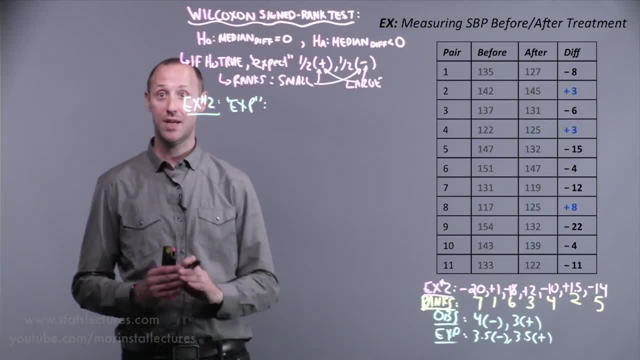 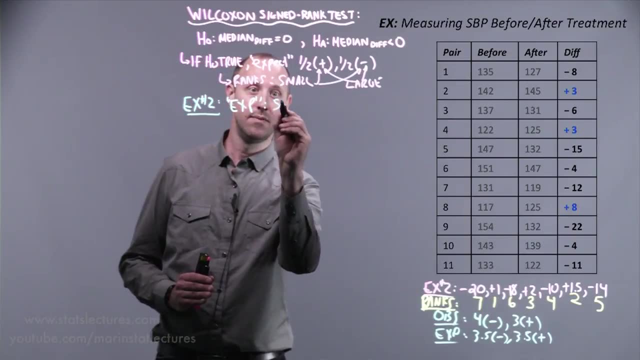 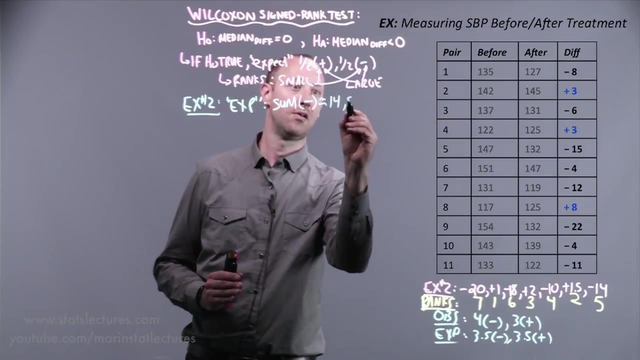 We're going to find the sum of those comes to 28, and we said we'd expect them to be evenly split amongst the increases and decreases. In other words, we'd expect the sum of the decreases to be about 14, and the sum 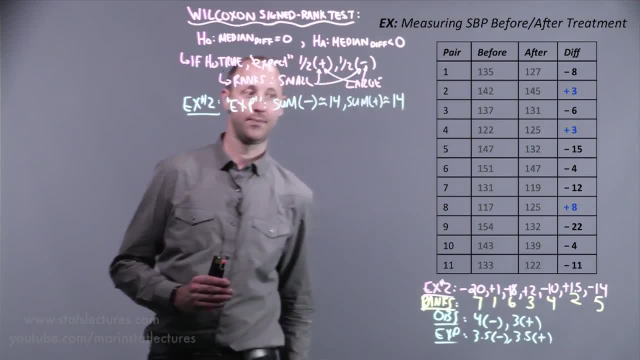 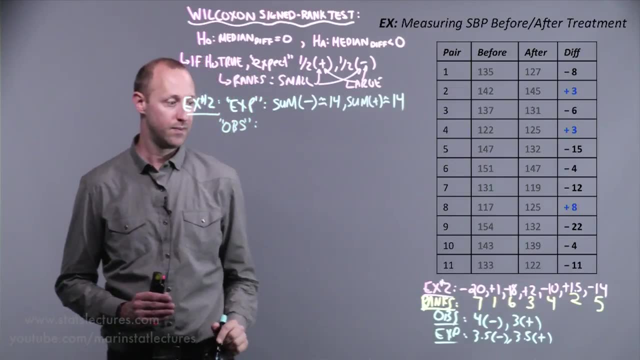 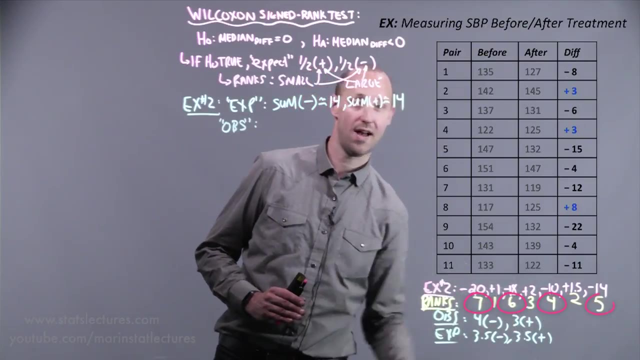 of the ranks of the increases to be roughly 14.. Now let's take a look at what we observed. in our sample We saw, for the decreases, they've got a rank of seven, six, four and five. So if we sum up, 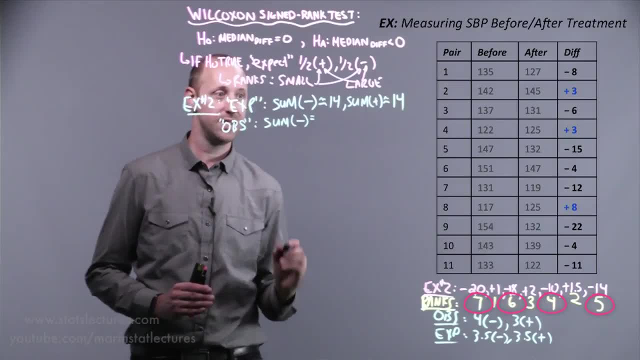 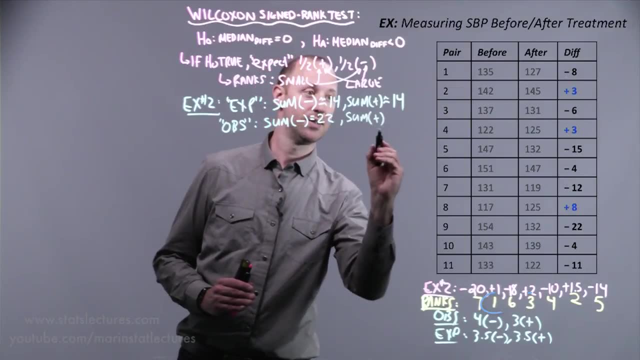 all of the ranks for the decreases, those are going to come out to be 22,. and if we sum up all of the ranks for the increases, those are going to come out to be six. So again, we can calculate a p-value here and that. 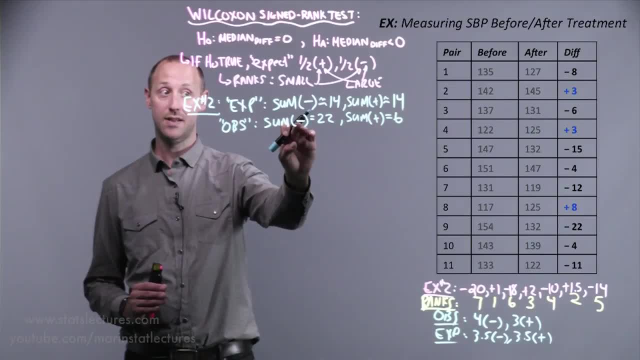 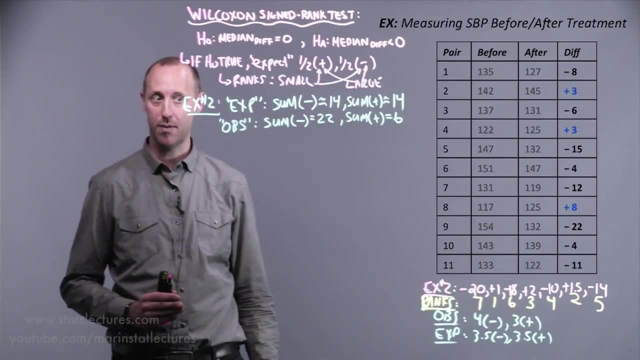 p-value tells us what's the probability of seeing, say, the sum of the negative ranks being 22 or more, if in theory, the null was true and it should come out to be about 14.. So again, let's write that here. 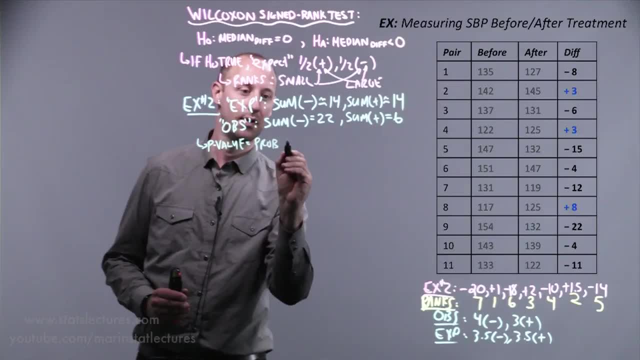 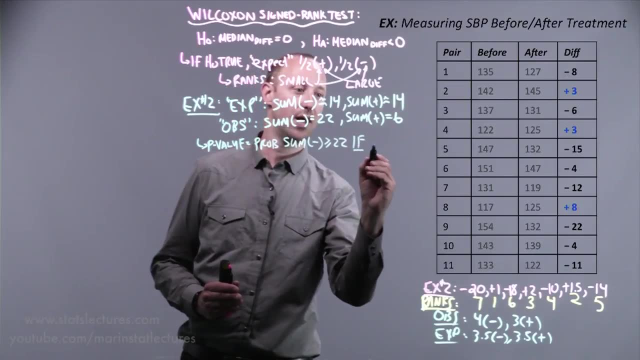 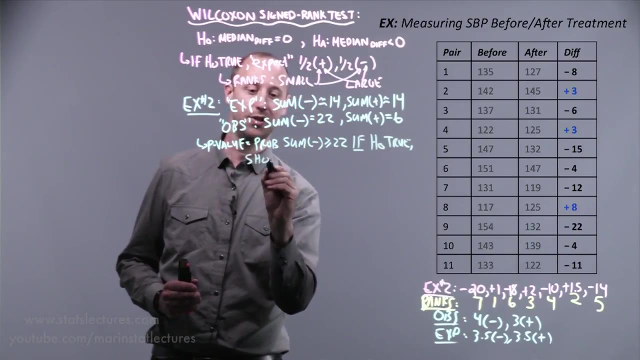 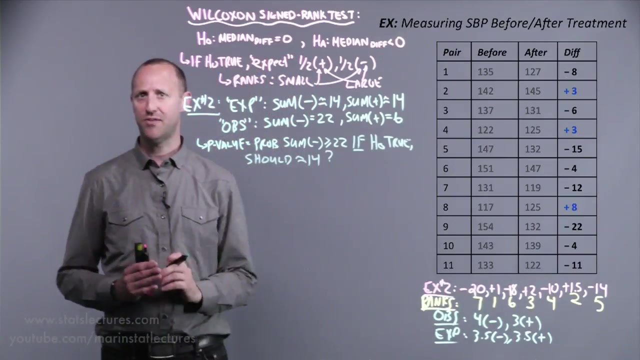 The p-value is going to tell us what's the probability that the sum of the negatives is greater or equal to 22, if in reality the null is true and it should come out to be about 14.. And again, there's tables to find those exact values. Let's not worry about the 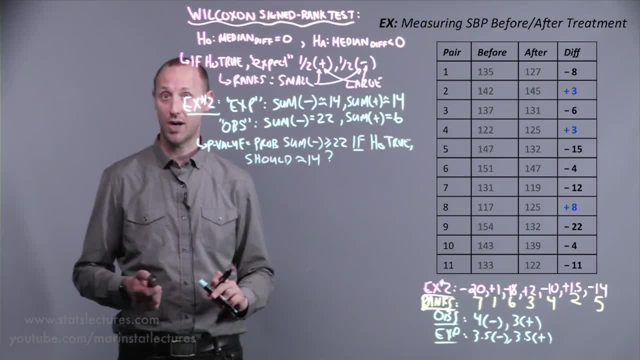 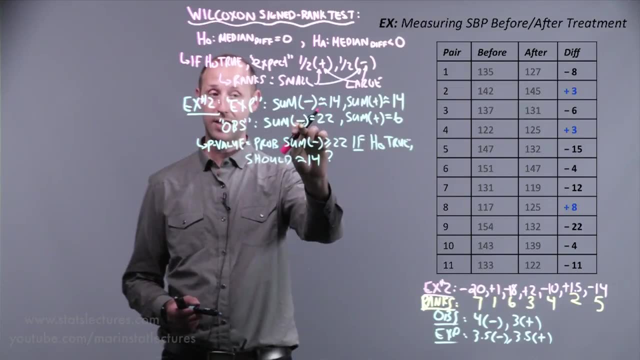 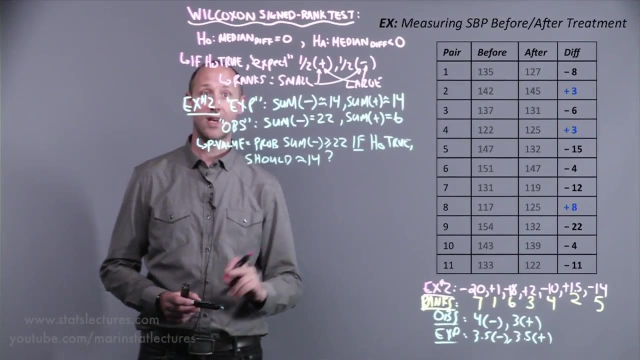 mechanics of it. Let's focus on the concept of what is this test trying to do So we can see. it's comparing the signs, the decreases and the increases, but also incorporating the ranks. Were the decreases large or small? Now let's get to looking at the larger example we have here. 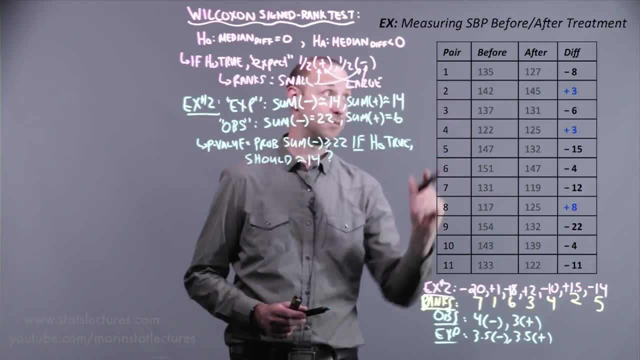 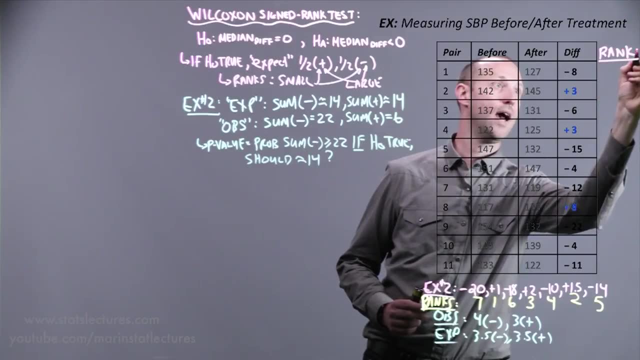 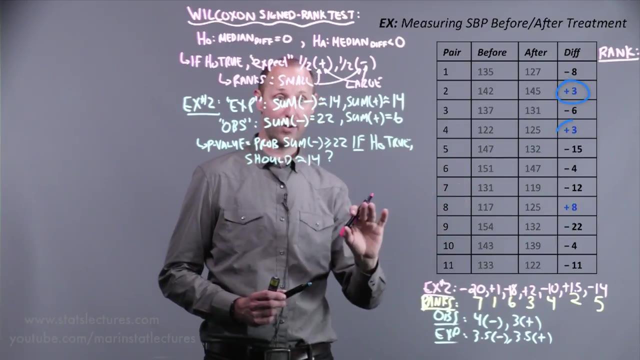 We can see that we have all these differences and over here, if we include the rank again, the rank of the absolute changes. if we take a look here, we're going to see that there's an increase of three and another increase of three And those are tied for the. 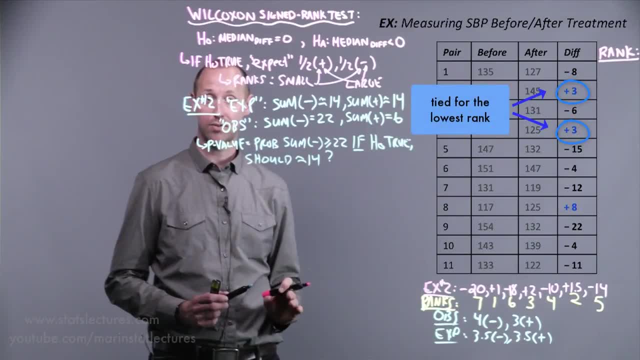 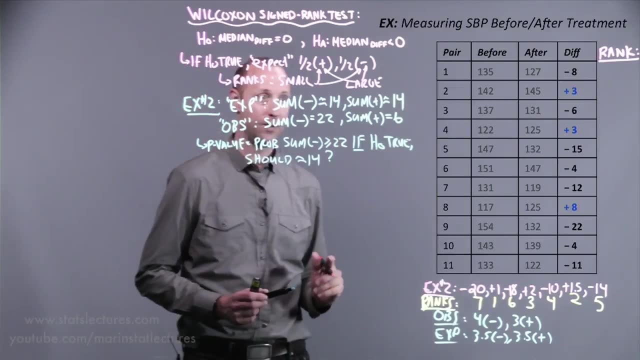 first rank, the first lowest rank and the second lowest rank. So what we do is we assign those the average of their share of ranks, So they're both going to be given the one and a half rank. So first we've got this one here and 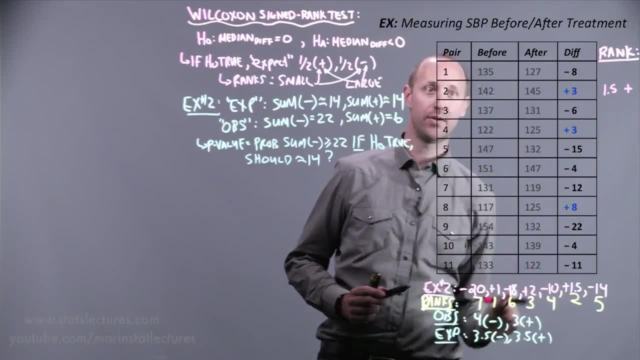 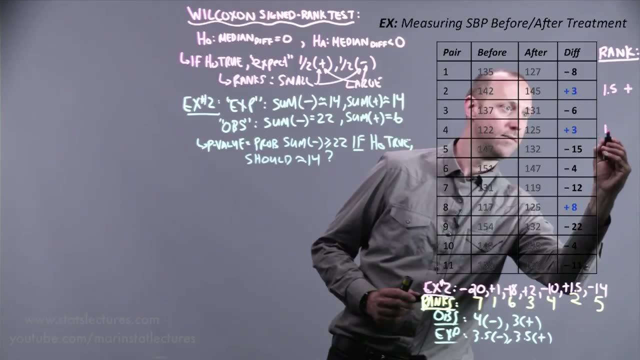 it's in the one and a half rank and it was showing an increase, So I'll just add that there. And then the other one we have here is sharing the one and a half rank and it's an increase, So I'll put a plus there. 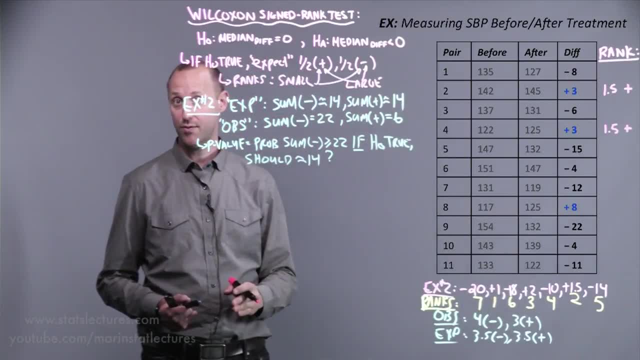 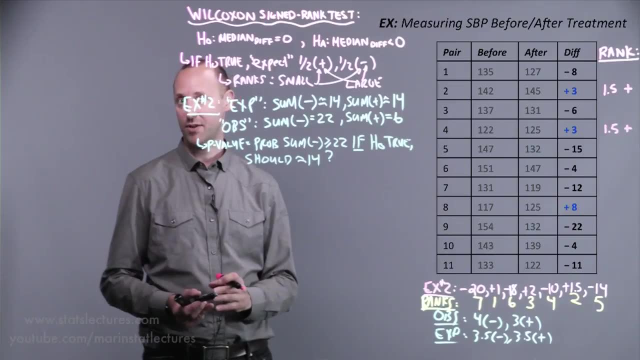 Then the next lowest ranks. there's a decrease of four and another decrease of four. So those are sharing the third rank and the fourth rank. So we're going to assign them the average of the ranks, the third and a half rank. That's right here. 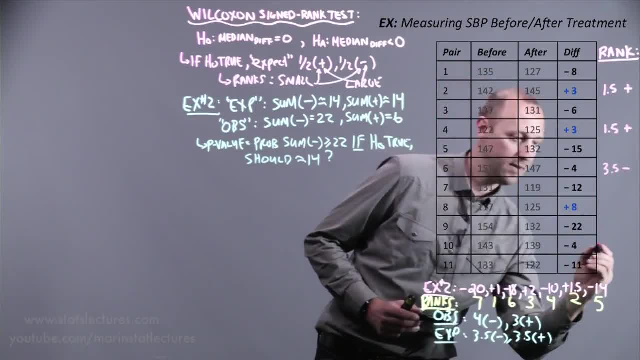 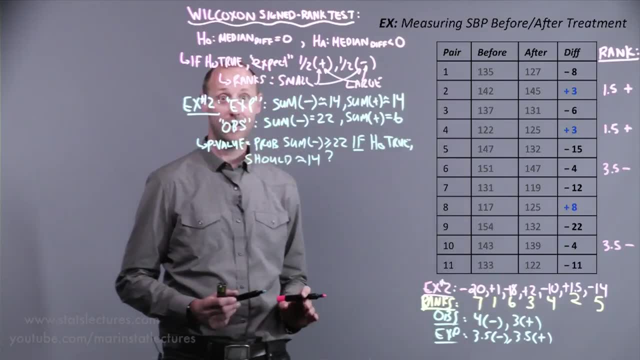 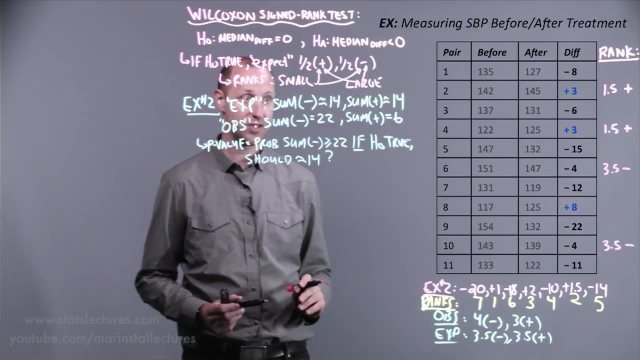 And it's a decrease. and then this one here sharing the third and fourth rank. After that, the next smallest change is the decrease of six. So this is sitting in the fifth rank, or the fifth smallest change. We can see that one right here. So again, that's. 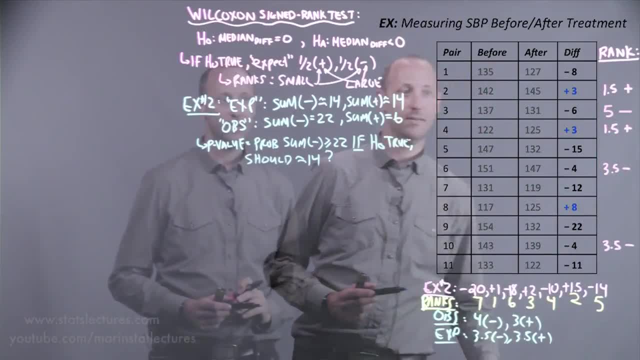 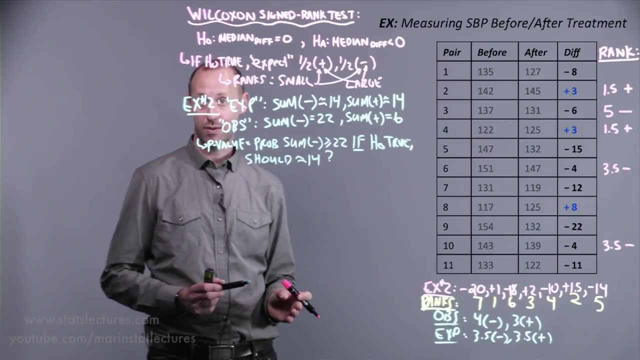 in the fifth rank and that was a decrease. Then we can say that there was a decrease of eight and an increase of eight And those are sharing the sixth rank and the seventh rank. So we're going to assign the average, the six and a half rank. 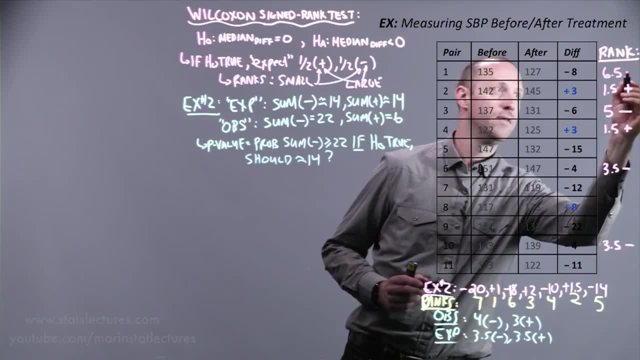 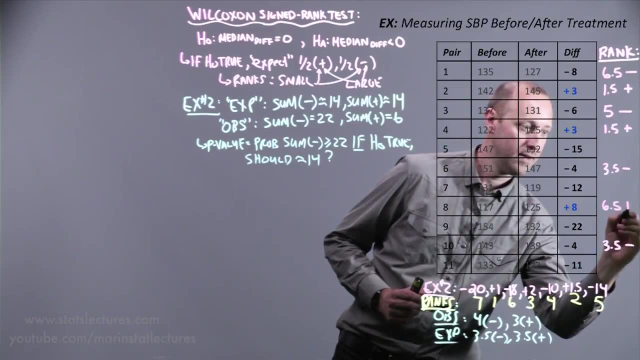 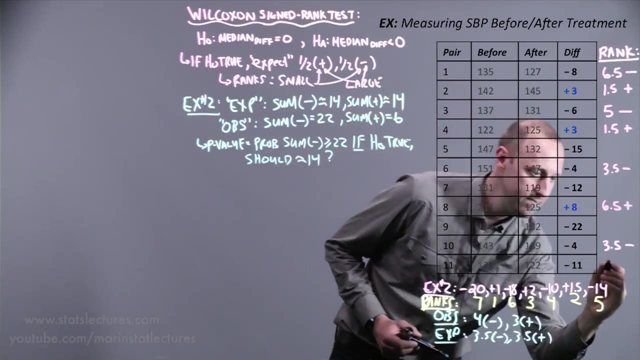 This one here is ranked six and a half, and it was a decrease. This one here is a six and a half rank and it was an increase. Then we can see: the next smallest one is the decrease of eleven, and that's in the eighth rank. 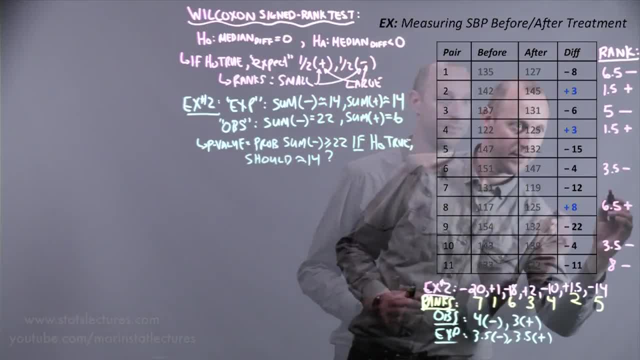 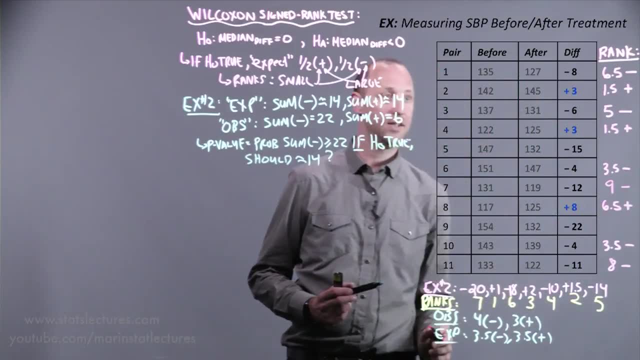 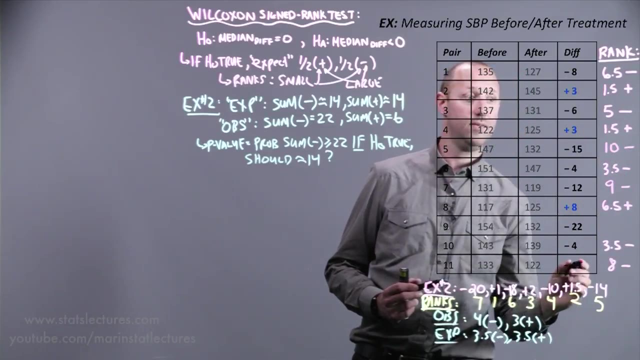 It was a decrease. Then the decrease of twelve, that is in the ninth rank and that was showing a decrease. Then the decrease of fifteen, and that's sitting in the tenth rank. That was a decrease. And then the decrease of twenty-two, which is: 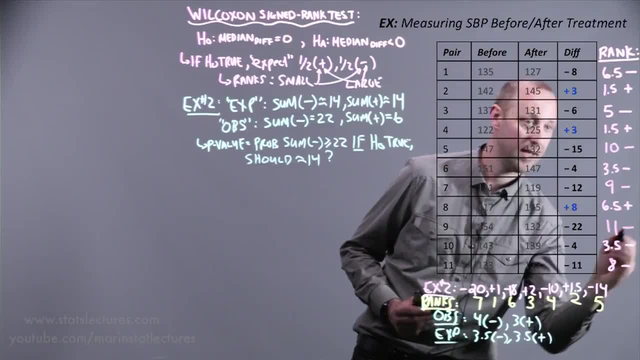 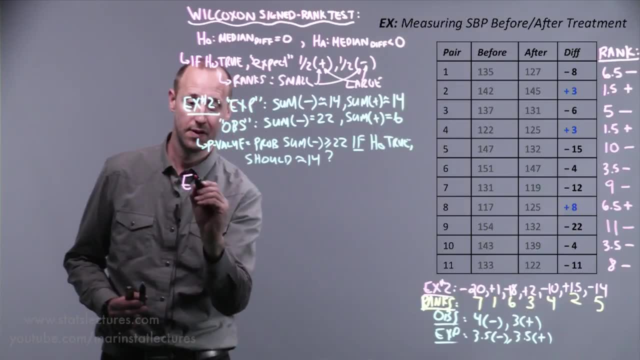 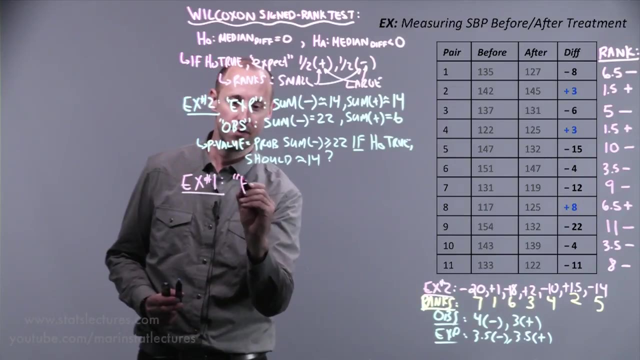 the eleventh, the largest rank, And again it was a decrease. So let's take a look at doing the same here. So this is what I'm labeling example number one. Now, first let's think about what we expect if the null is true. So if we sum up the ranks, one plus. 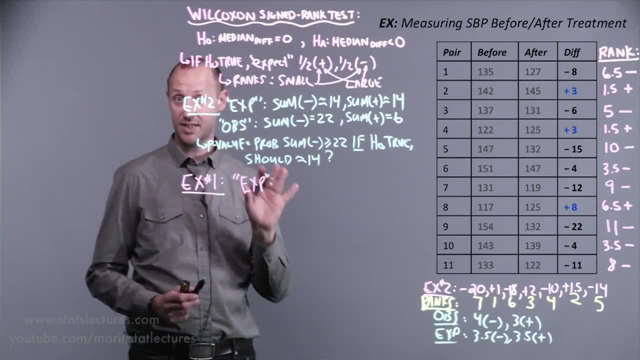 two plus three all the way up to eleven. that's going to come out to sixty-six, And if our null is true, we'd expect about half the people to show a decrease, half to show an increase, and we'd expect the large and small ranks. 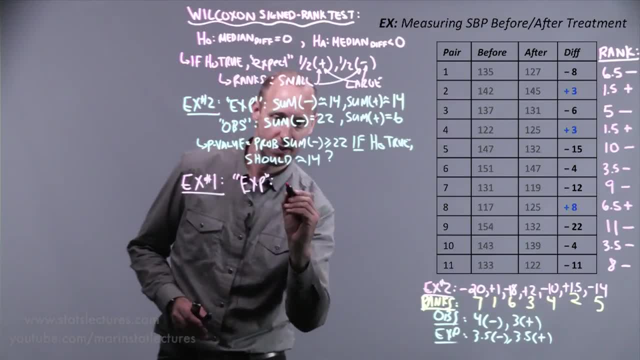 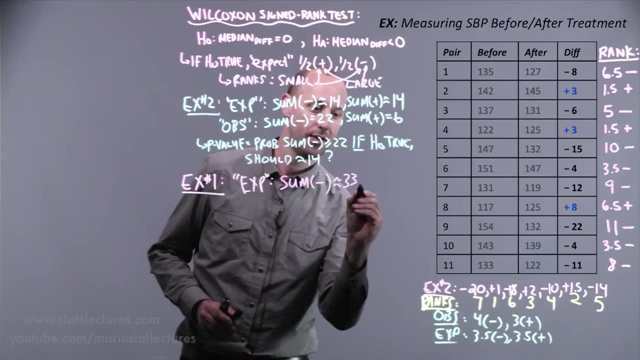 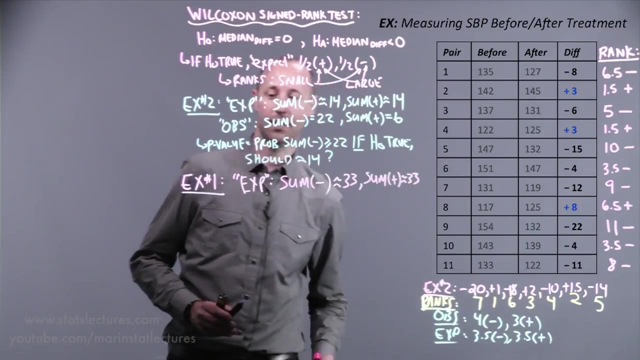 roughly equally balanced. So we'd expect the sum of the decreases to be about thirty-three and we'd expect the sum of the increases to be about thirty-three. Now, what do we observe in our sample? We actually did this for our observed data. 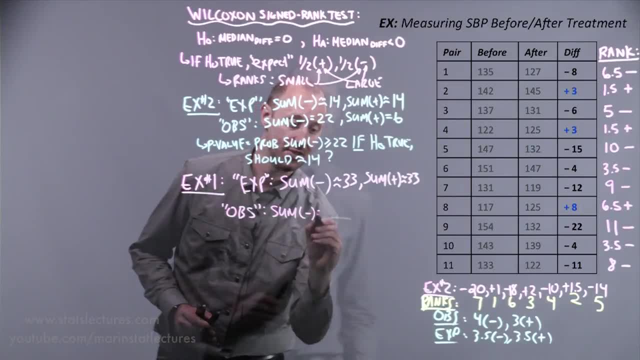 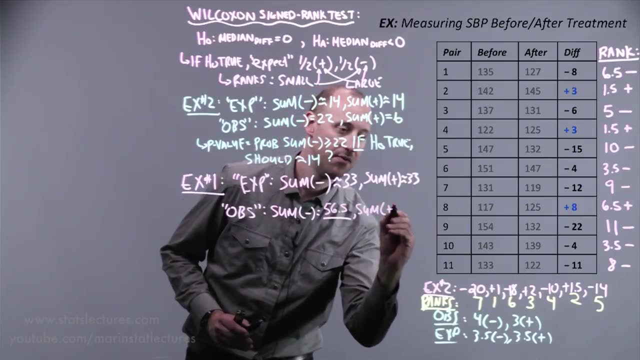 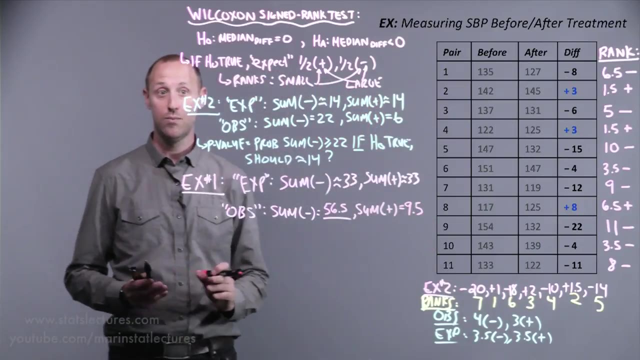 We saw that the sum of the decreases, that's going to come out to be fifty-six point five, And the sum of the increases came out to be nine and a half, And so, again, we can calculate a p-value that tells us what's. 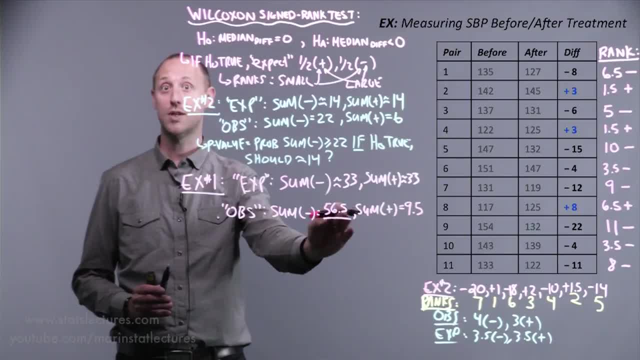 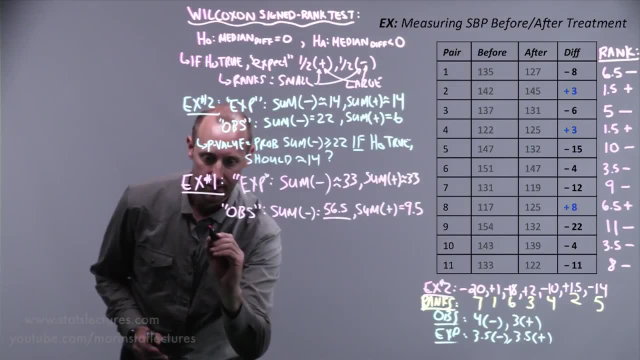 the probability of observing what we did in our sample, or something even further from the null or more extreme, if the null is true, and this is what we'd expect to see, So we can calculate p-value Again. this tells us: 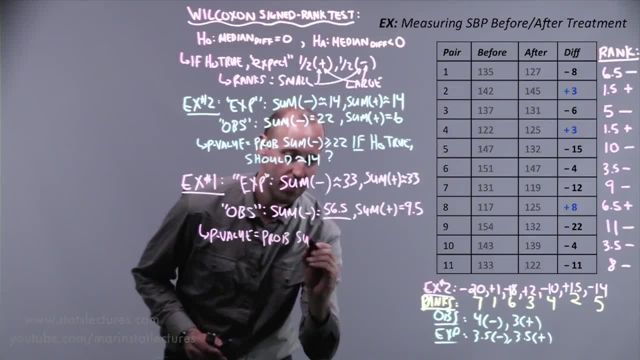 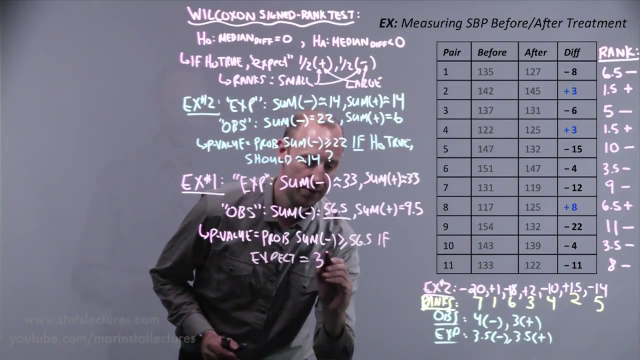 what's the probability of observing the sum of the negatives being greater or equal to fifty-six- point five- if in reality the null is true, and we'd expect that it should come out to be roughly thirty-three If you work this out. so if you take this data, put it in software and ask it to. 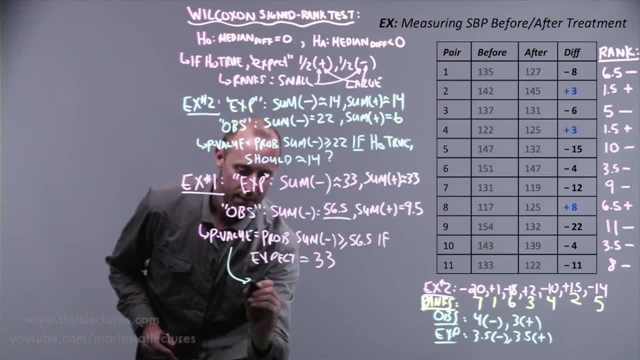 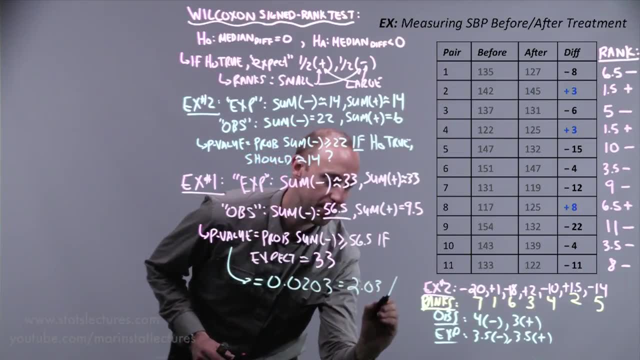 do the Wilcoxon signed rank test, you're going to find that the p-value here comes out to be point zero, two, zero, three Or two point, oh, three percent. And again a reminder: this is for the one-sided test. If you did the two-sided test, 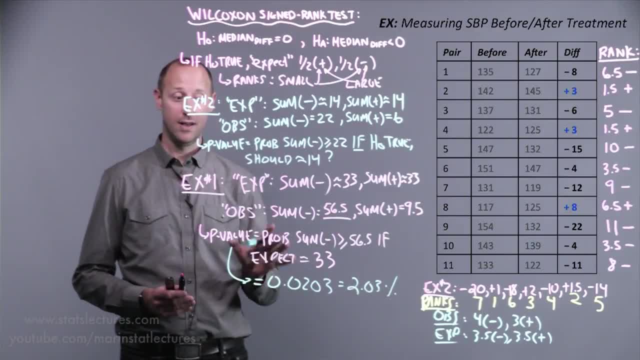 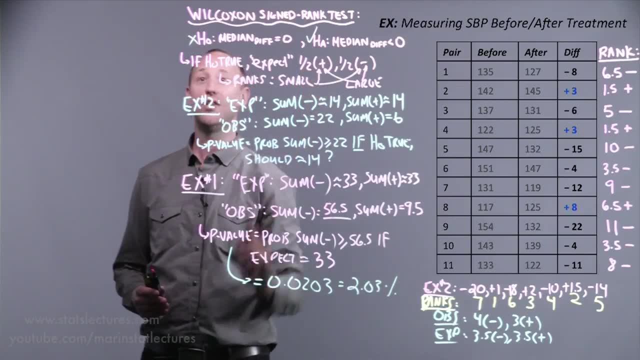 it would be double. We're going to end up reaching the same conclusion. Since our p-value is small, we're going to reject our null hypothesis. We reject our null. we have evidence to believe the alternative is likely true. The median decrease is less than zero. 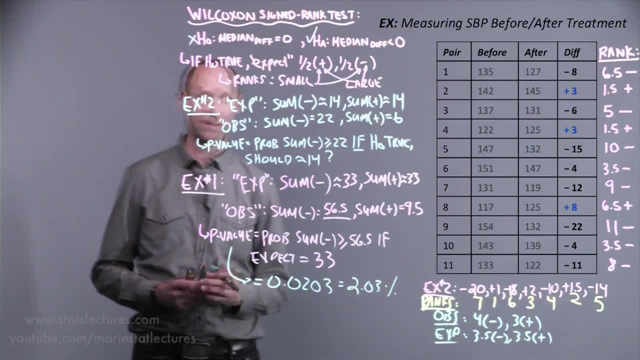 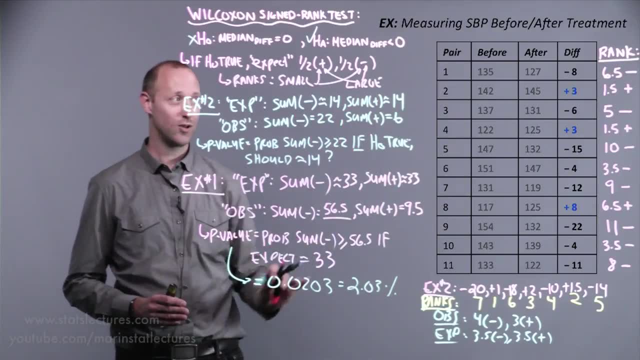 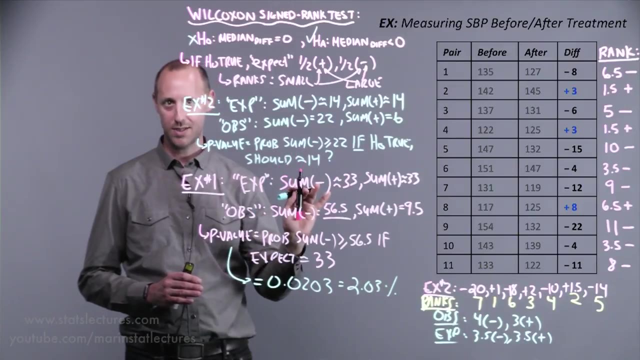 People are experiencing some decrease after treatment. So again, just a final reminder: doing this stuff by hand is not important. It's a distraction from your learning if you try and focus on how do I calculate all these ranks, sum them up and so on. What's important is the concept. 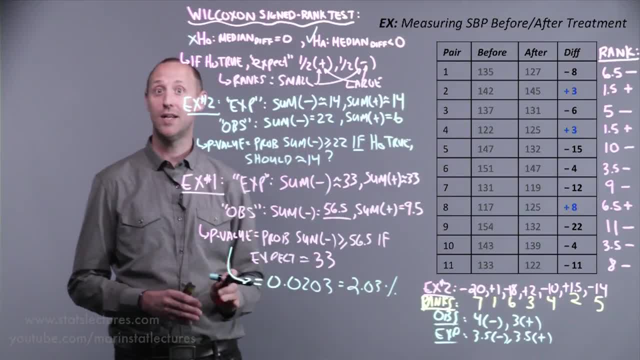 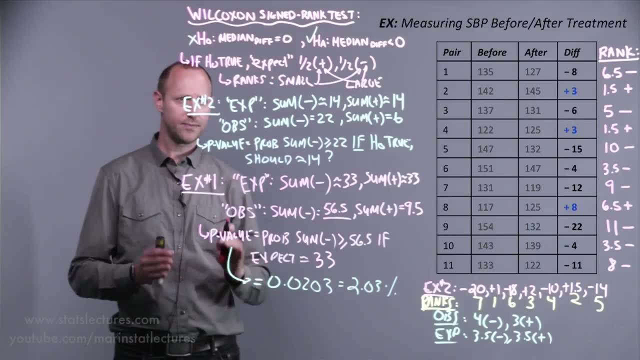 and understanding. how is the non-parametric approach trying to get at the same question that the parity test or the parametric approach did? All the different non-parametric tests you can encounter, the parts change slightly. the underlying concept is generally the same. 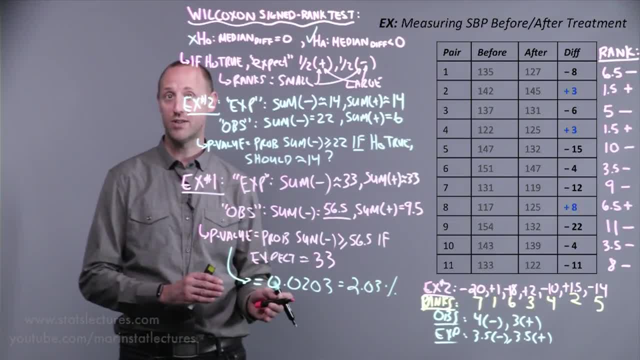 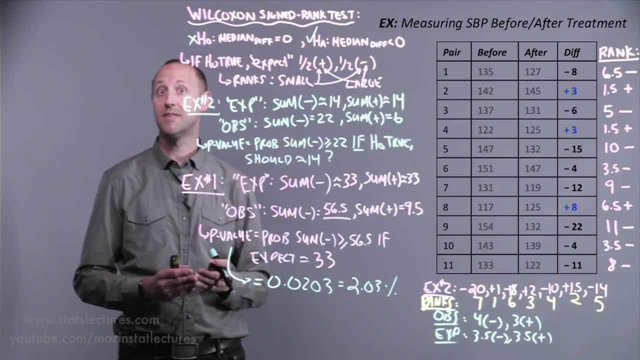 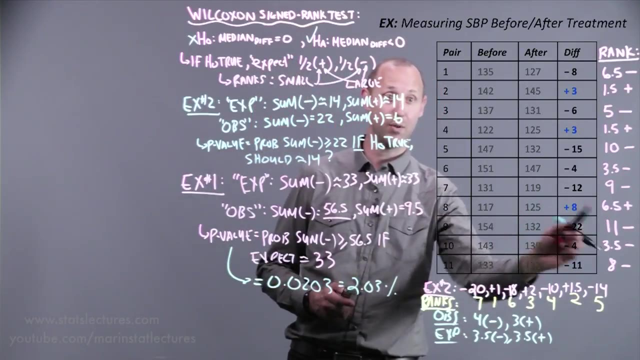 They usually work with ranking observations rather than the numeric values themselves. There is gains and losses to these. By ranking the observation, the gain becomes less sensitive to outliers, Whether the largest change was a decrease of 22 or a decrease of 42.. 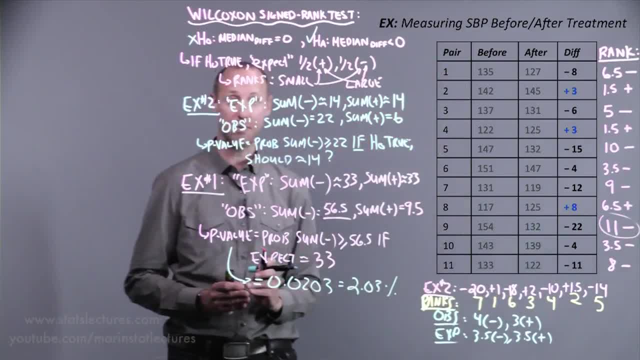 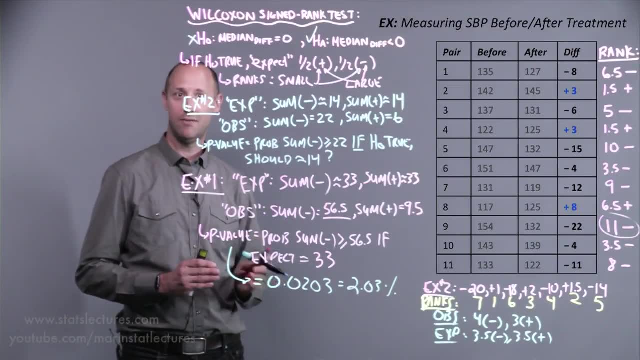 Either way, this is going to be the largest change, So it doesn't become sensitive to an outlying value or an extreme value. So in some way that's a gain. A negative of using ranks is it throws away some information, Seeing a decrease of 22 or a decrease of. 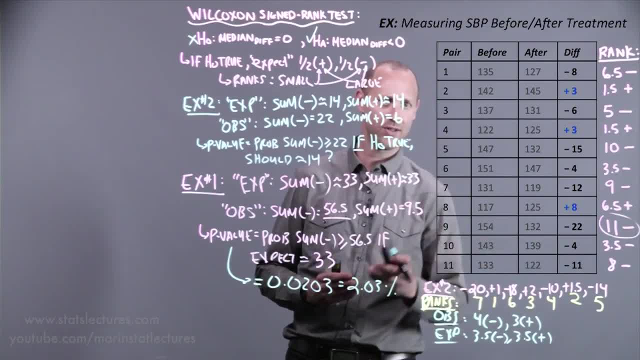 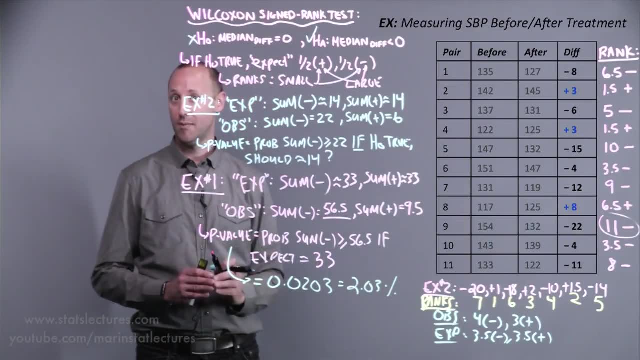 say 26,. those are slightly different pieces of information. The decrease of 26 might be a bit more informative or a bit larger and you're kind of losing some of that. So gains and losses to these non-parametric approaches versus parametric. But just a reminder, they're a slightly different way of getting at the same problem.